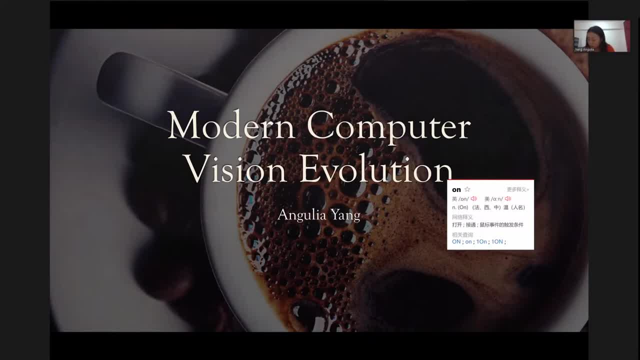 So, if I mean you know, you've been following Angulia. she's a frequent speaker on women who code forums And we have shared the state somewhere in January where we discussed about debunking AI myths- about, you know, robots and machine learnings and AI failures and successes. 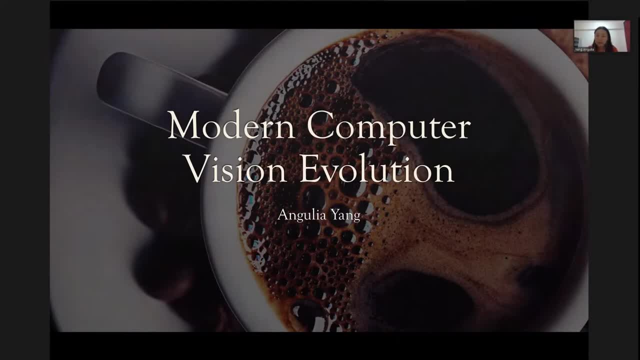 And she has received her education from NUS with a master's in computer science. She has four years of experience working with machine learning, computer vision and uh. she's also developed several vision projects, projects including medical image analysis, video analysis, surveillance and autonomous driving, so which is, like you know, the 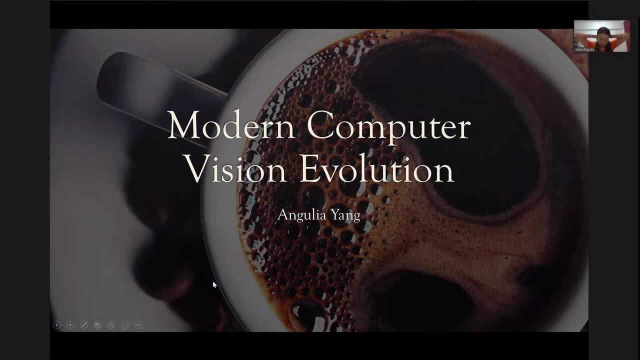 robotic and self-driving cars which are of that most importance nowadays. and she also, you know, is of the opinion that there is no single best ai approach that works for every scene. so she's actively exploring more innovative methods or to deploy and to get the ai to work. 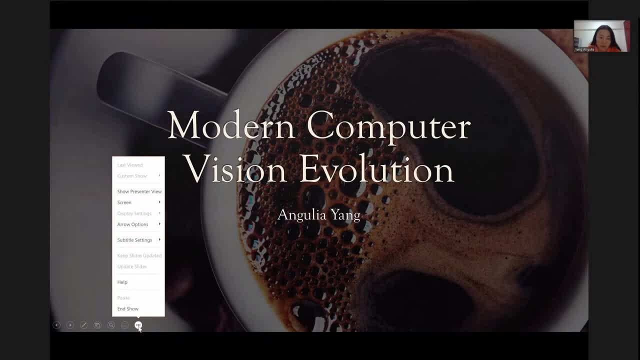 and with that, you know, we are all set to listen to angolia's take on computer vision today. so, yeah, it's all yours, angolia, okay, thank you. thank you, priyanka, and thanks for inviting me. uh, today's, uh, this year's a tough year. hope everyone is okay and stay safe, okay, so. 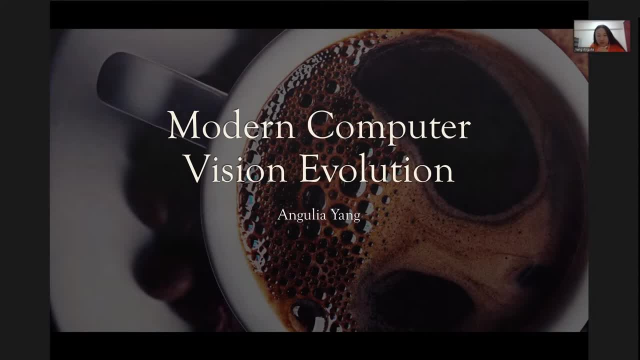 you uh, since my major uh research topic is highly related to computer vision and i've been working in industry for years. in this area and beyond that, i'm also part of the researcher and also keep track of all the updates in this faster growing community. so today i'm gonna share you with some um my understandings and also sharing with some uh. 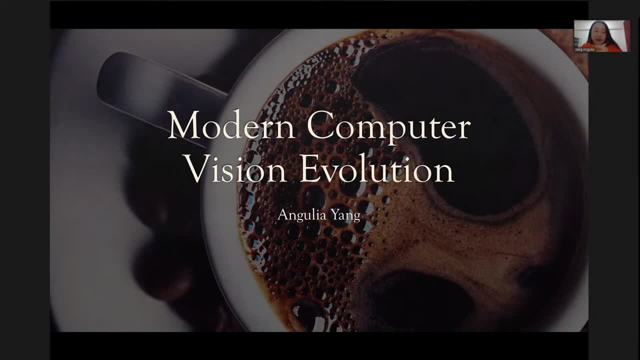 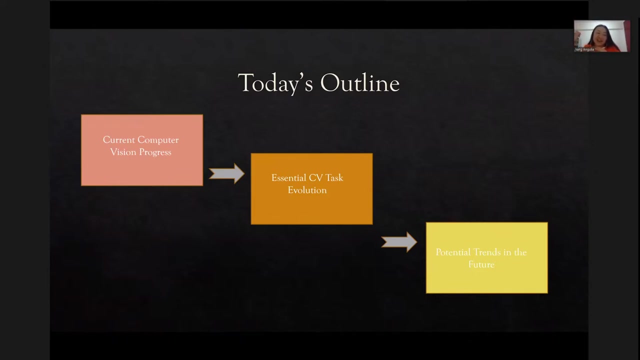 evolution of these computer vision techniques and also about the um, future trends, uh, trends of this computer vision research and also application. uh, of course i know every computer vision research is going to be about the future of computer vision, and i'm going to show you the data, all the knowing part on what's going on that way. and so, moving on to the next, 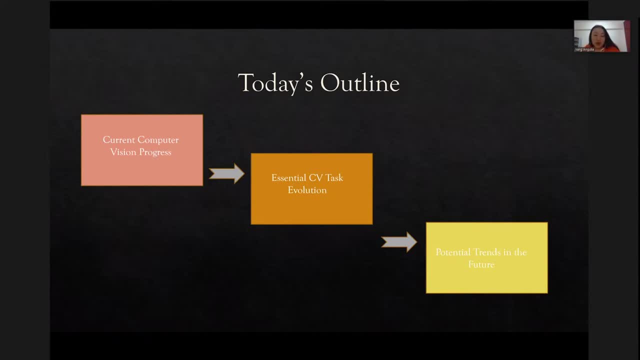 lesson uh on the computer vision class, and uh, on this interesting topic about um, early decision generation, on decision planning, and uh, the really good story about um, like how much my. So I will give everyone an overview of how the current computer vision, the community and their research, their application, grows and how about the progress for now, like 2020, right, 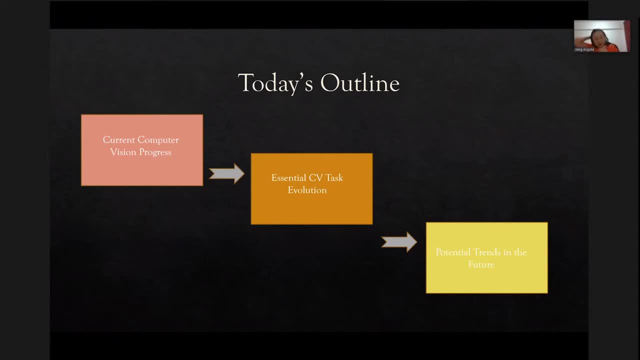 And then I will try to go a little bit deep into the specific tasks, like for the essential tasks like image classification, object detection and also image segmentation. these are all the basic but essential tasks in this vision community. With the knowledge I won't go very deep. 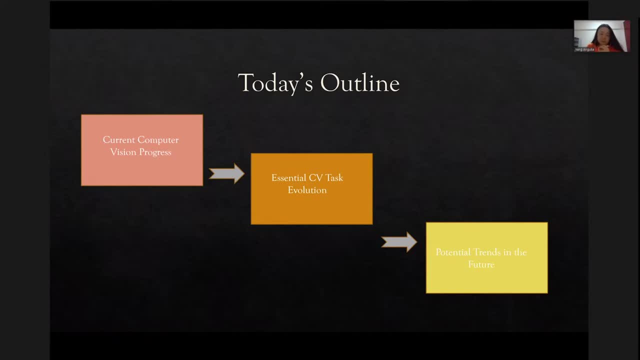 I won't go into the mathematical way or into very detail, but I will give you a blueprint of how these tasks evolve and how the correct characteristics was added within this process. Then we're going to discuss and maybe talk about the potential trends in the future of this computer vision. 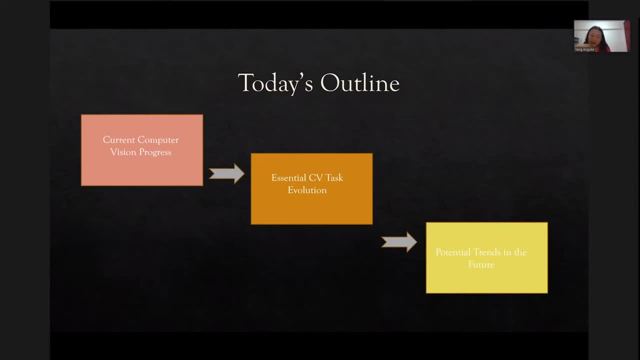 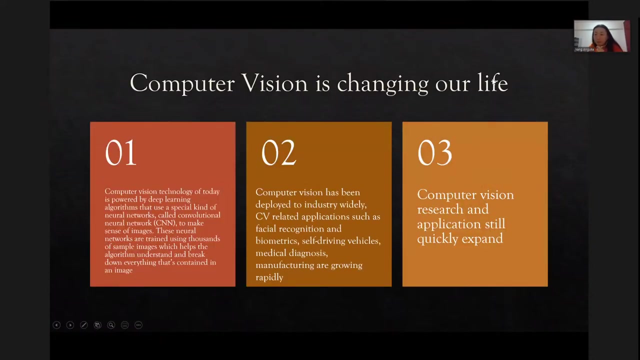 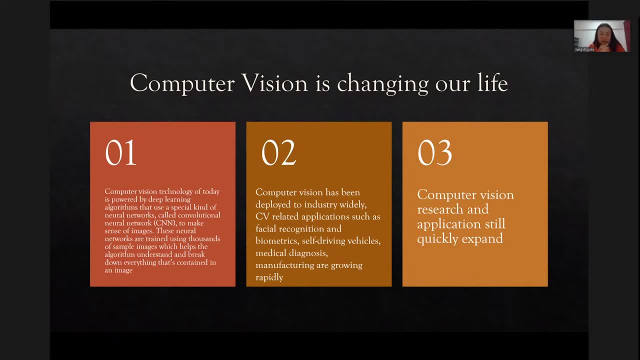 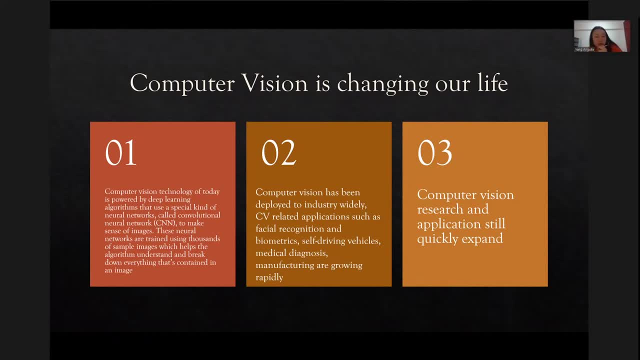 More commonly used is convolutional neural networks. With such algorithms, we can more effectively make sense of these images And those networks are trained to use. are trained based on thousands of input data, samples, the images so-called, and such images helps the neural networks to be more accurate, to be more specific to your task. 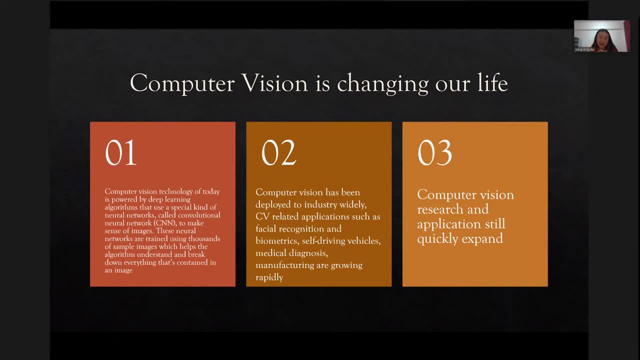 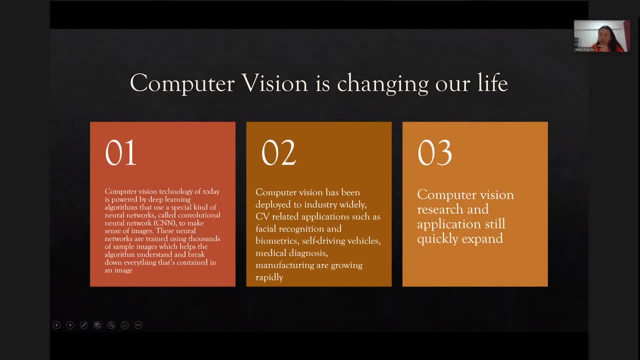 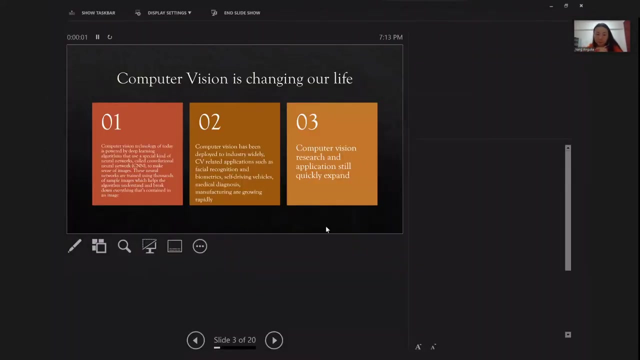 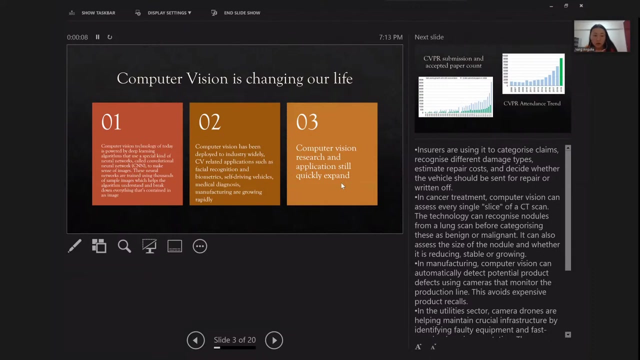 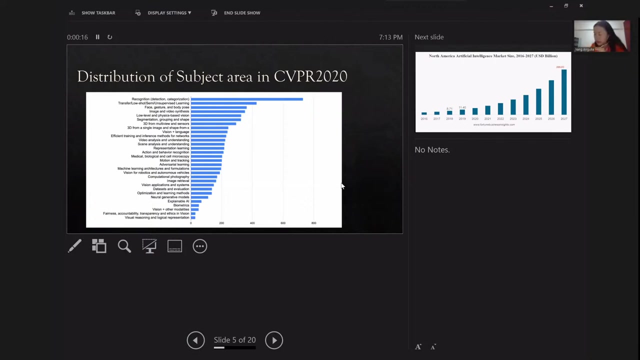 And tier. now. this community has been widely applied into the real world life but beyond. they are still quickly expanded in other research areas or other applied domains. Okay, so first let's take a look at this top conference of computer vision research. 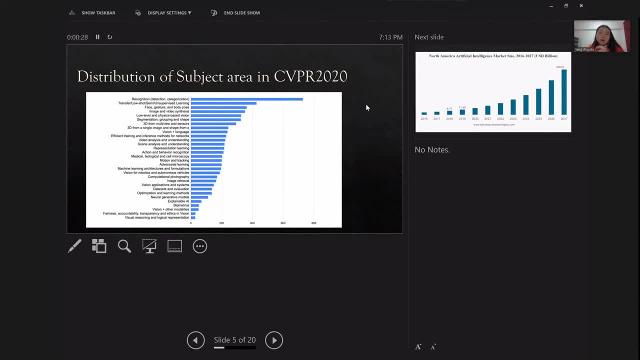 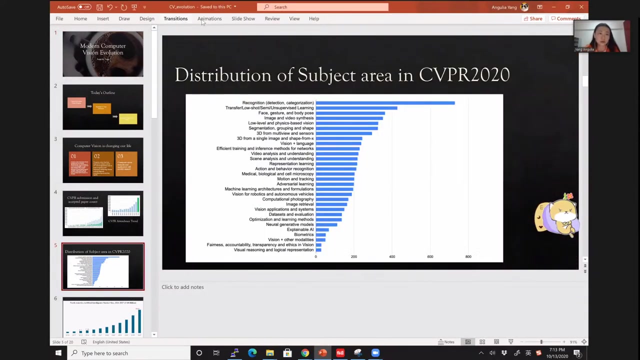 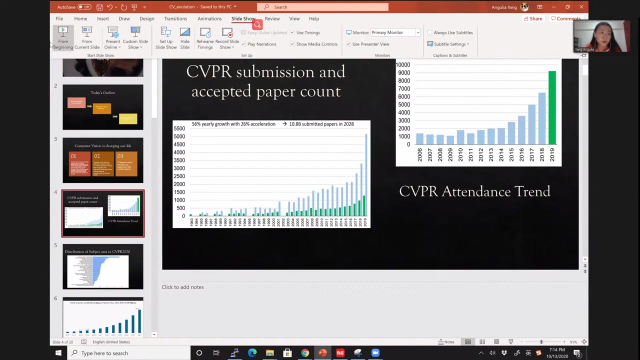 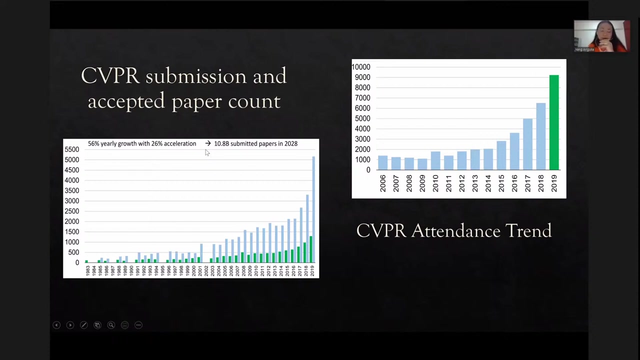 For computer vision research. the top conference will be the CVPR so-called. so Computer Vision and Pattern Recognition. What are you trying to get done, Angulia? Yeah, I'm trying to project the presenter mode. Okay, Let's continue. 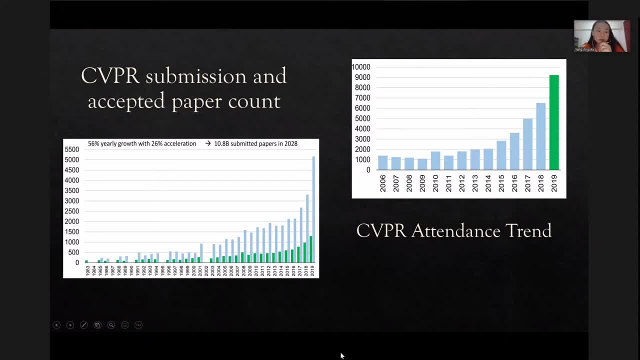 Okay, so let's first start with academic world. For academic world, the CVPR is the top conference for this computer vision research, So the state-of-art research and ideas, innovations will be published. Okay, So the top conference will be published. on this conference proceedings: 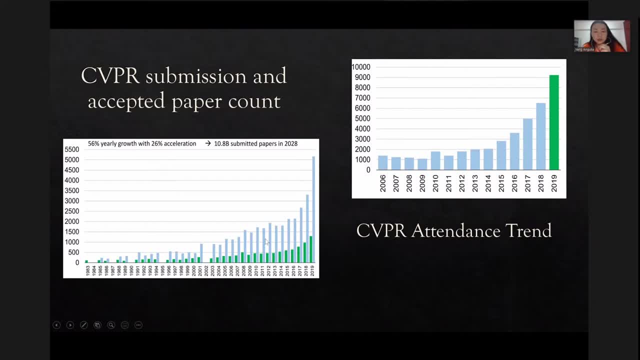 And we could see since 2012,. after the occurrence of our deep learning decades, there'll be a directly increase for those paper submission And we could see that people are very passionate About this area for the computer vision research and also for the attendance trend we could. 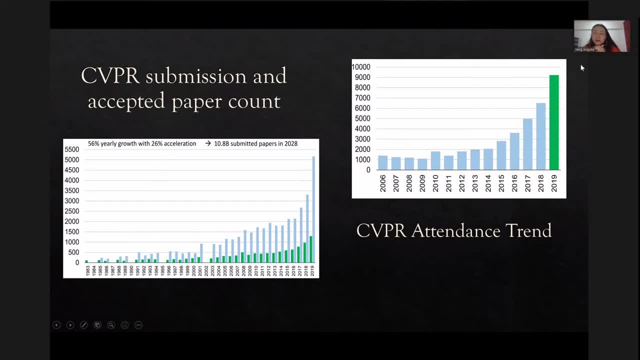 also see this directly goes up in the past 10 years. So still there are many, many people are trying to get involved into this AI world or into this computer vision. Okay, Yeah. So I think it's very important for the computer vision community to enable their applications. 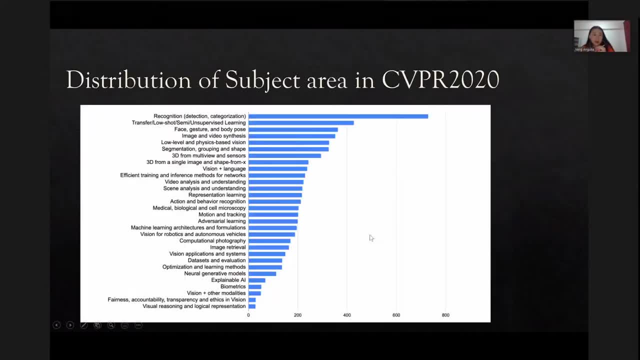 or enable their research. And in recent years we could also summarize sort of the topics in the CVPR and we could see like: So now we could see some sort of trends in the current research for the first. of course the recognition problem is always the first problem in the computer vision. 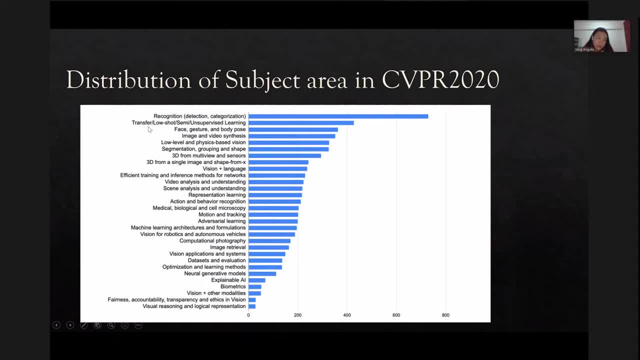 But in recent years something interesting trends I see and like to share. one is like the transfer learning. Oh, so-called transfer learning, Okay, So we know that the same semi-supervised and unsupervised learning are getting noticed more and more often. 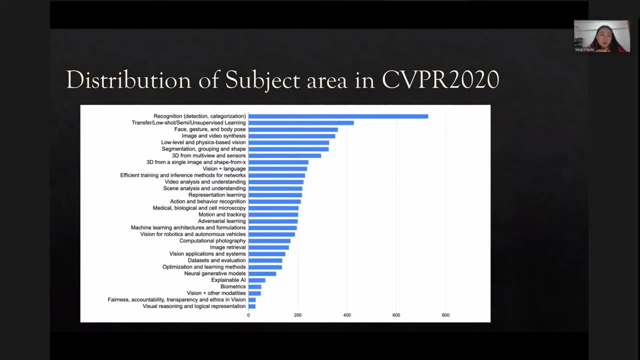 Since, like the Like we all know for the traditional, like imaging that, and the CIFAR-10, those existed big data sets- has been trained well and now people are wondering, like, how better we could be like a human learn, say, like for for our traditional deep learning. 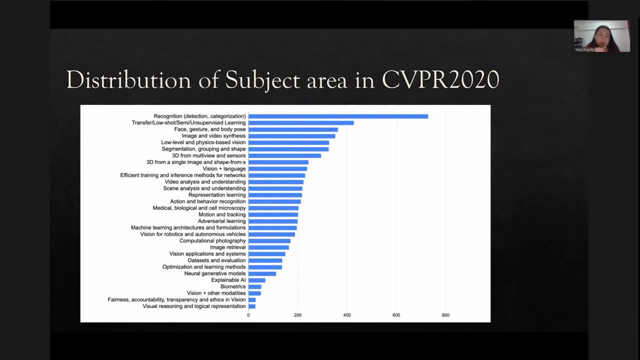 neural networks where you thousands of images as input feeding. but for people- people when learn to recognize an object, we don't need to thousands of samples to recognize right. so now there's a trend is to get more close to the way of how our human brain works, and this is one very interesting trend recent, in recent years in 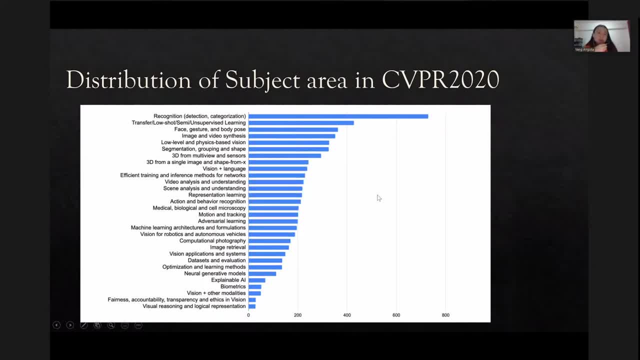 recent uh, the current research, and on the another part is a 3d, 3d data with some sensor equipment equipped and enabled in recent years and with also uh, some open public uh data set has been published, um, now 3d is also another trend for uh for this year's research, say like from previous. 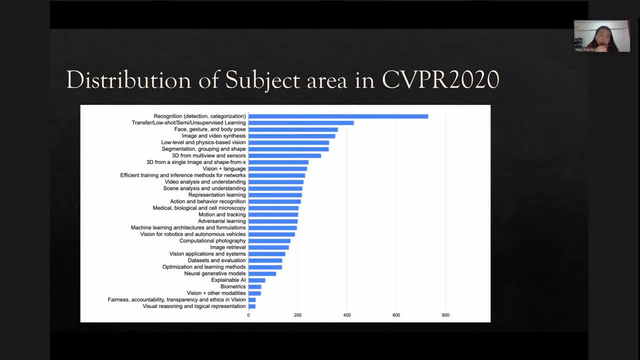 years. we are working on only 2d the plane, but now we'd like to know the whole view of these objects, which is a higher level understanding, and beyond that, we know we noticed. uh, there's also another very interesting topic arise, which is a fairness and accountability. 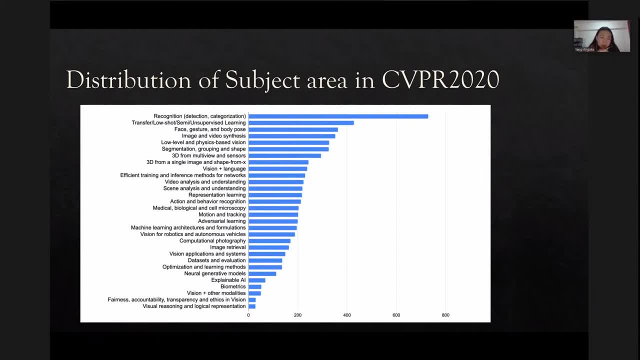 and transparency ethics in the computer vision, because we see, like in medical image analysis and uh the famous autonomous driving, which all uh involves some law issues or ethics issues about this uh technique and also the laws, the rules. so how do we justify and how we better utilize this ai to empower our life rather than? 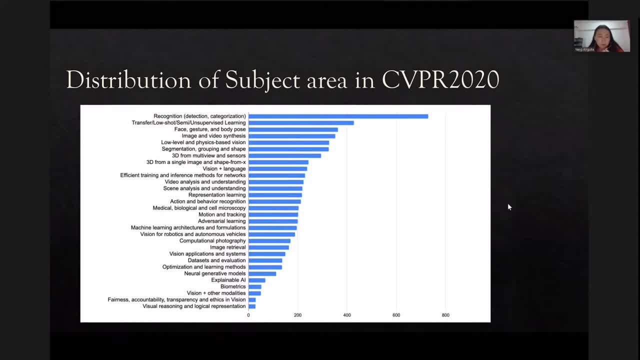 being abused. so this is also an key issues of this uh um, of this topic, so i'll so i'll show this. basically, transitions from the academic worlds and this academic words also give some uh indication for those uh partitioners who are newly joined this um community and would like to contribute more and like to ex explore more new things, this can be. 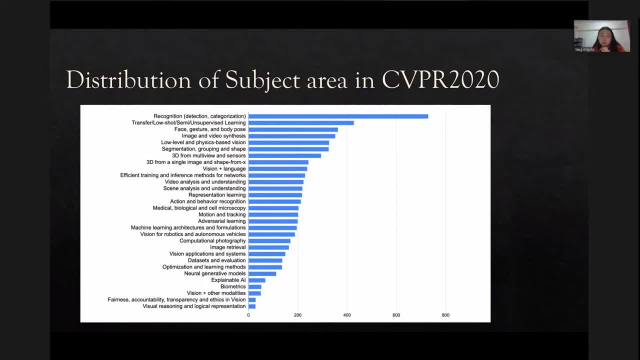 sorry and this can be a very good uh trends for you to explain and to see how you can um, how you can use uh the existed work to ex expand your, your own works. and this is basically from the uh academic research, their um, their current status and all their current focus, and beyond that, we also could see that 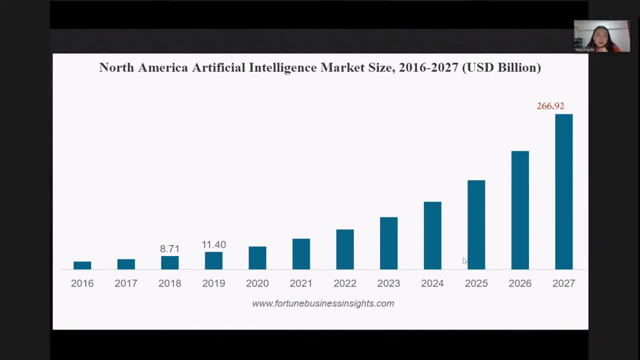 for their uh from the business prospect prospect. we could see uh since last year, last year, last year in north america. in north america the artificial intelligent market has already reached uh 11 billions and according to the fortune free cast tier 2027 there there will be 260 billions of market of this computer vision. so we could see there are more potential. 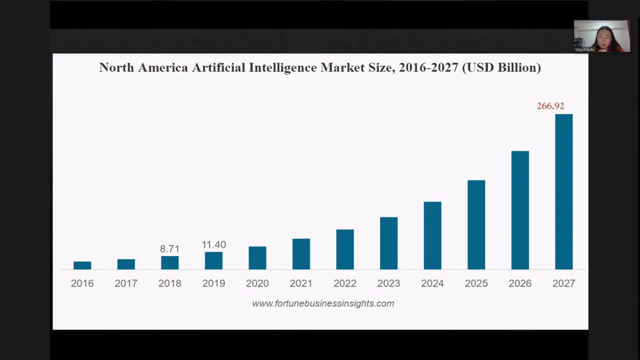 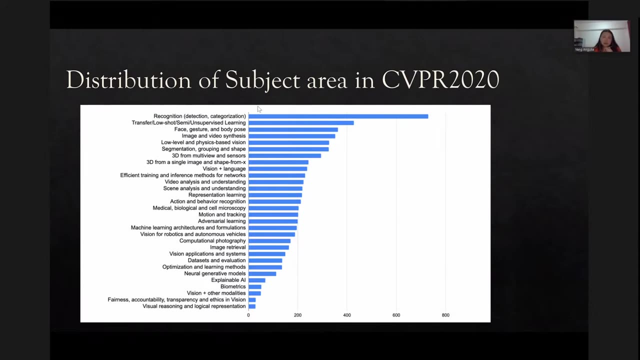 opportunities for more opportunities in um there expectation, um uh in this community and also in the business prospect prospect for now, some, some, uh, some like some. some essential tasks or basic tasks like image classification and object detection and object segmentation. later i will, i will cover that, but uh, yeah, this is been解体ed太多目前后 intervening operation operatori. i will cover that. but uh, yeah, this is a puisque des deceased kokoreский. 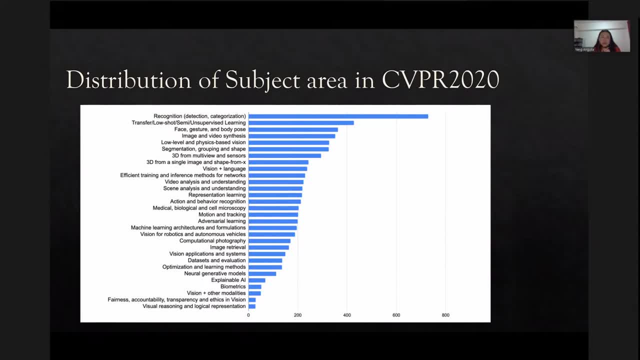 chez the von. i recently moved to japan because something was not implemented, it was imposible, and there were still some feeling, many memories of music and such of a correcte calciumом, biologico적인 essential tasks. now has been kind of we say, mature. 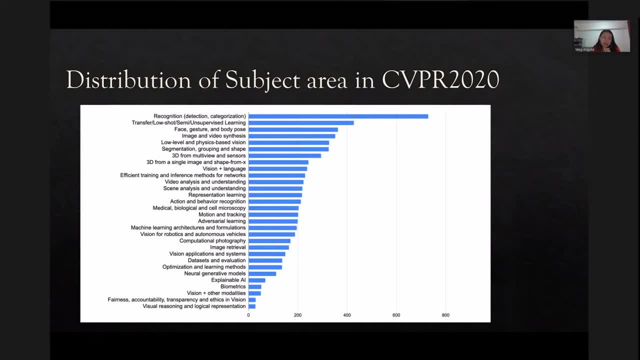 and being successfully deployed into our daily life, Like our face recognition, our traffic surveillance, analysis software sort of things. But some, like we call those semi-supervised learning and about the 3D learning and sort of like adversarial real learning about the security of this computer vision. 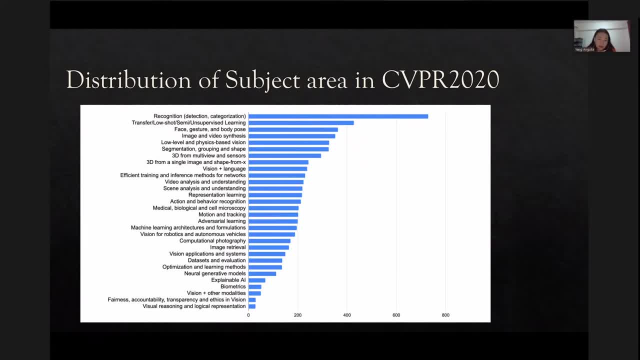 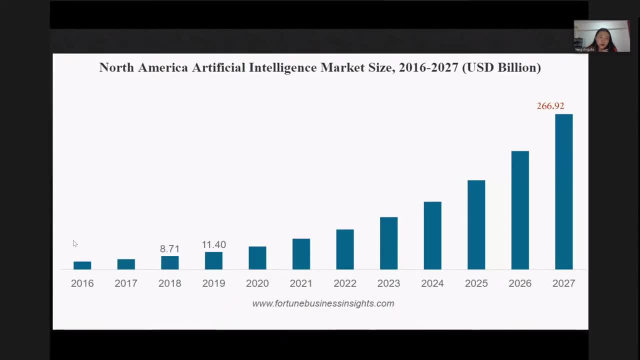 about vision tasks. These are also the faster growing, faster growing business for those who want to make the computer vision research into a product or make use in industry. So here's a trend, So we could see there are a lot of expectations there in this area and in this domain. 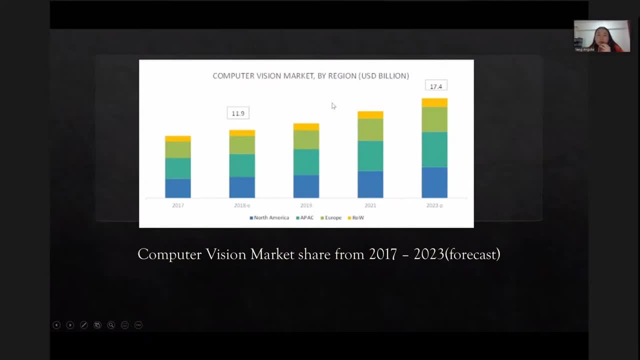 So further. we take a closer look like, say, for the specific computer vision market by region, we could see for North America and the Asia Pacific, and also Europe. The three parts takes the dominance of the computer vision market And in 2018, there'll be 11 to 12 billions. 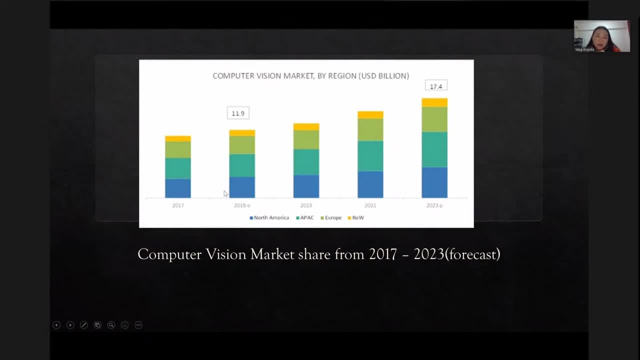 in the whole world market And, according to this, three places share sharing almost equal 30s to this whole market and the tier 2023, there'll be also increasing numbers And also during this year for the COVID-19,. the computer vision has been also utilized. 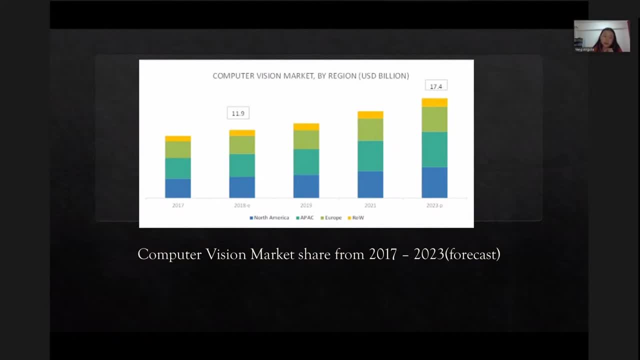 for diagnose: the lung MRI and lung CT images to diagnosis how the patient goes, how their illness goes, how their blood pressure goes and so on, And how to justify whether they get affected. So this domain do have some more potentials to increase. 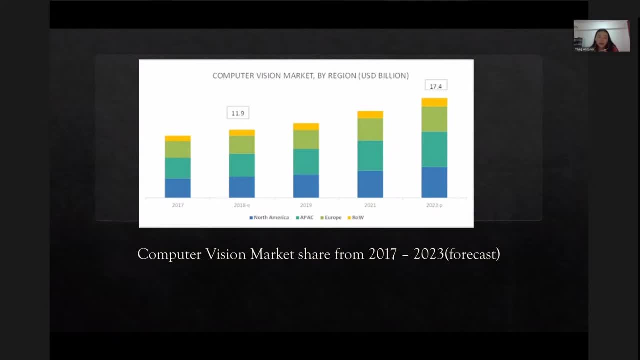 So this is basically an impression for those who are new into this community- for I'm sorry, So this is from both the academic world and from the business aspect- of how the current computer vision is going and what's the progress we could see. for some now, 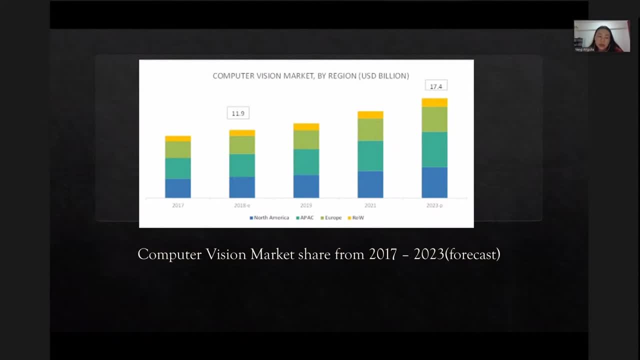 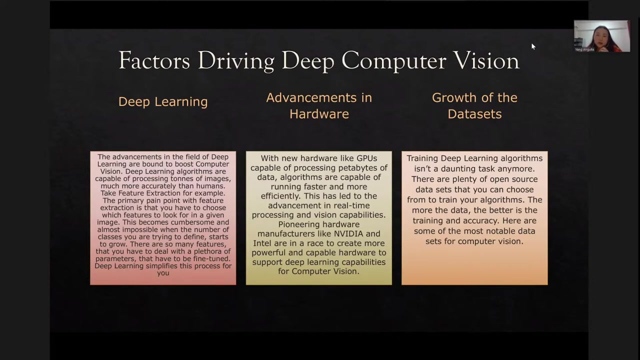 now the computer vision in both industry and academia world. we have a strong basis but still there's a lot of space to explore and for for us to start our business and or to start our new research topic and and what are the key factors about drive in driving the deep con computer? 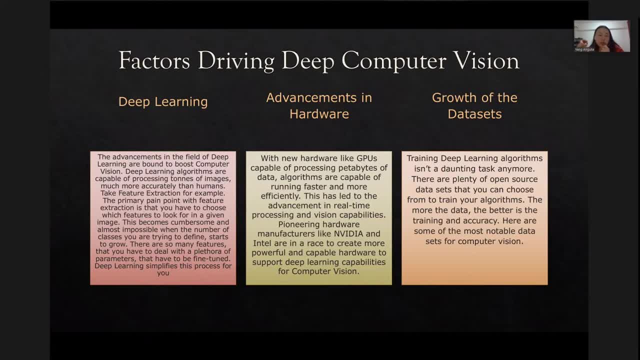 vision going. I'll say there'll be three key factors. One is the deep learning and the. The second is the advancements of the hardware, so-called the GPUs, And the third is the growth of the data sets. So we start with the first. 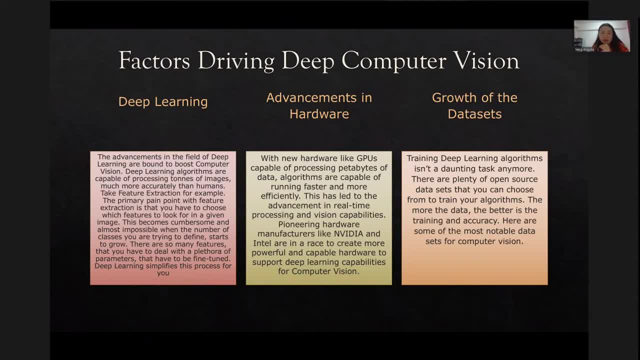 Deep learning enables the very first convolution networks into a powerful classifier in 2012 in the large-scale image classification competition. So this one is the multilayer neural networks, the capability of it creating a nonlinear mappings from the input to our target, The mapping and for the 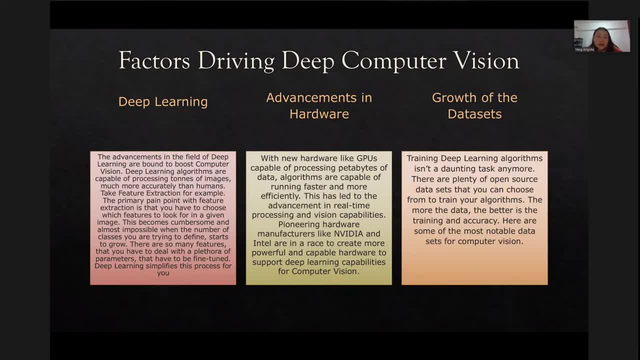 Complicated hyperplanet created has enabled the current computer vision progress. And the second is also with the help of the GPU- comes out Because we all knew like the initial idea of this convolution networks- has been occurred as early as in 1989. But with the new hardware like GPUs, 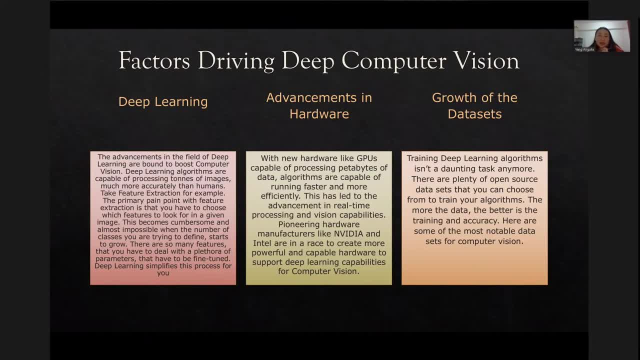 And for now even TPUs. right, they are capable of processing gigabytes or petabytes of data algorithms and do more efficient the metric computings, And so we can running our so-called training faster and more efficiently, And also it makes lots of application. 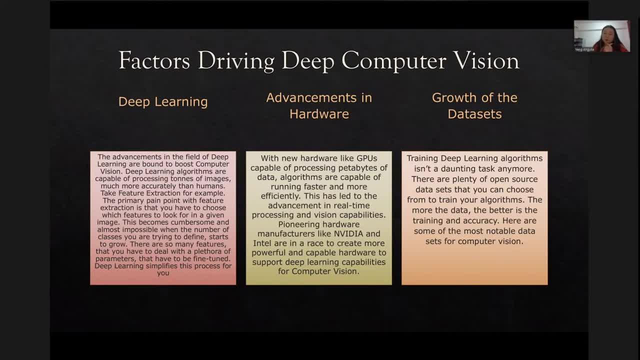 Into reality. So now, like for the object detection or classification, we can all realize the real-time processing, And the pioneer hardware manufacturers like NVIDIA and Intel are also in their race to create more powerful and capable hardware to support the future hardware development. 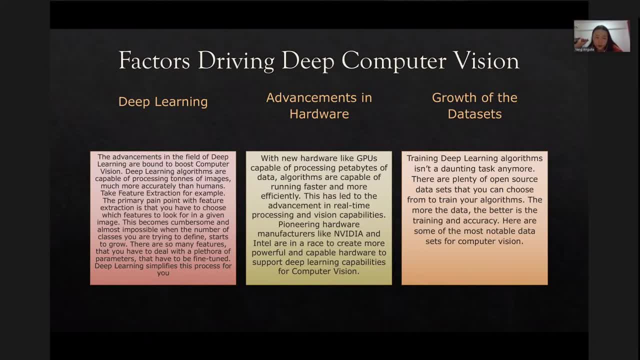 And so we can running our so-called training faster and more efficiently. And also it makes lots of application And so we can running our so-called training faster and more efficiently. the future: AI development And also in computer vision And also in computer vision, because computer vision in a way is also 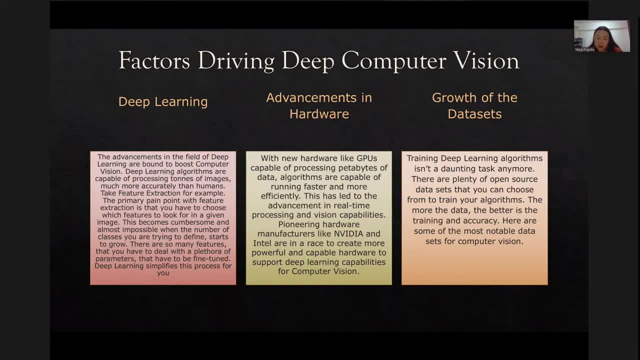 requires Lots of computing resources. since now we're upgrading from the past images resources to the video resources, the availability ofст Noel partner- The amount of data we could У Delete want to keep it up of GPU- is also another great backup for the deep computer vision growing. 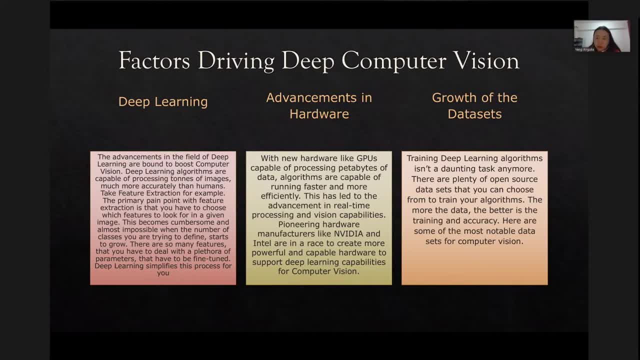 And the third part is about this community. Also, the growth of the data sets Because of the public data sets, makes like numerous images available. So the algorithms, the deep neural networks, different architectures are generated out of it, And this one is also thanks to many like research institutes. 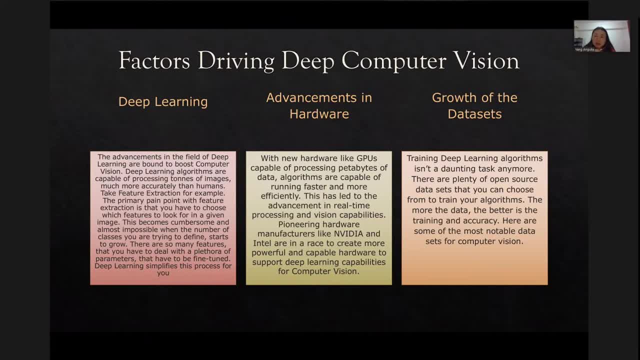 and companies. they contribute their times, they labeling the data and they release resources to the community. And also in the future we will need more real world like data sets, contributed into the research and into the application as well. So with this, three factors accelerated. 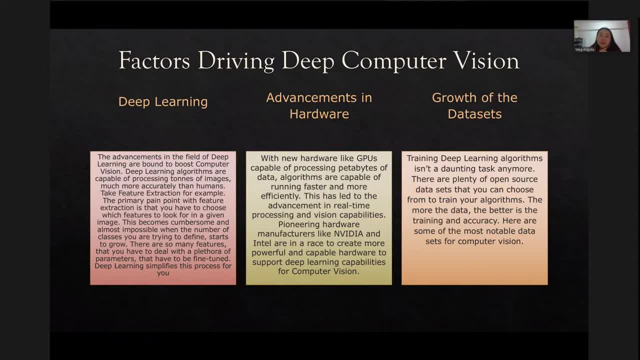 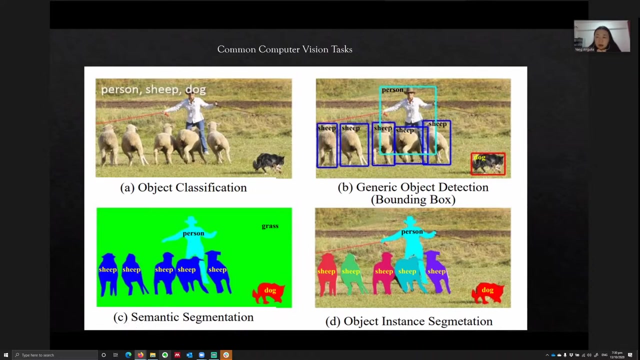 I think that creates the current deep computer vision, this community and this progress. So this is basically, I think from the overview, part of my understanding on the computer vision and it's deep learning. So in the next subsection I like to discuss some essential tasks because I know there are a lot of. 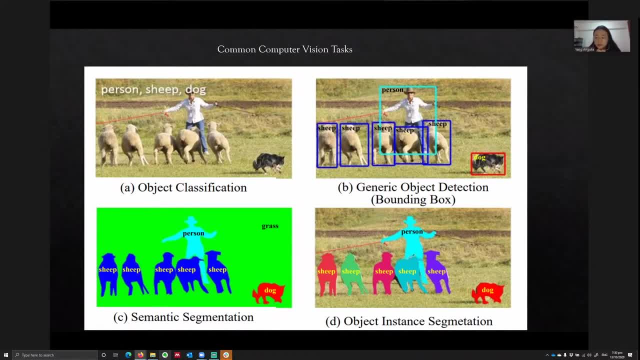 advanced topics like generative adversarial network or 3D detection, or the adversarial learning and also autonomous driving. But most of these tasks, according to me, they are based on these essential tasks and these essential tasks give the milestone of this deep computer vision. 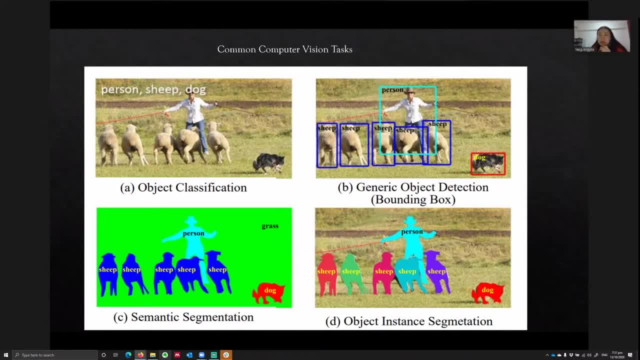 That's why today I'm gonna cover, like the object classification and the object detection with some semantic segmentation. I try to cover these three we call very basic task in the computer vision community and try to cover the three and some semantic segmentation. And then I'm gonna also cover some of these three. 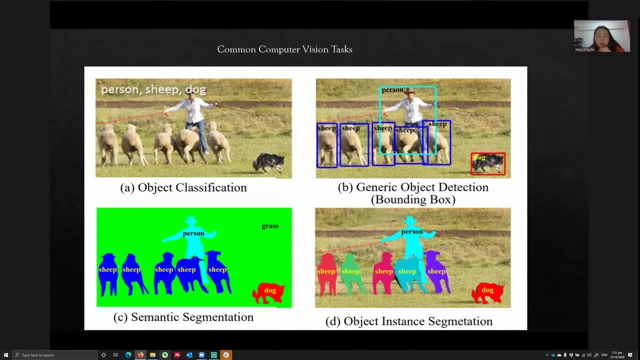 in the computer vision community And then I'm gonna also cover some of these three in the computer vision community. So I'm gonna take a moment to just talk about the evolution of these three tasks, to make you better understand how these tasks evolves and how the deep neural networks evolve. 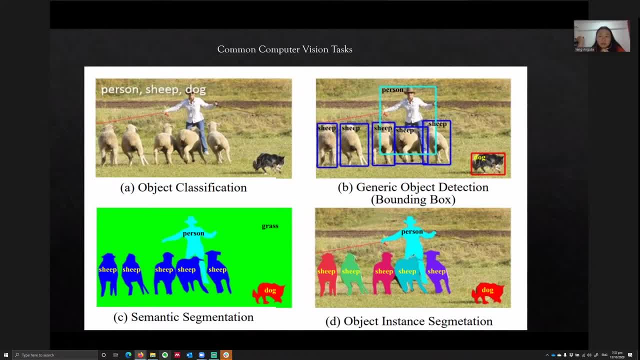 and how the deep neural networks evolve and become the current stage, And then we can further discuss, based on the existing works or based on the existing research and application, what are the potential um trends for for our future uh exploration? so start with the very basic. one is: 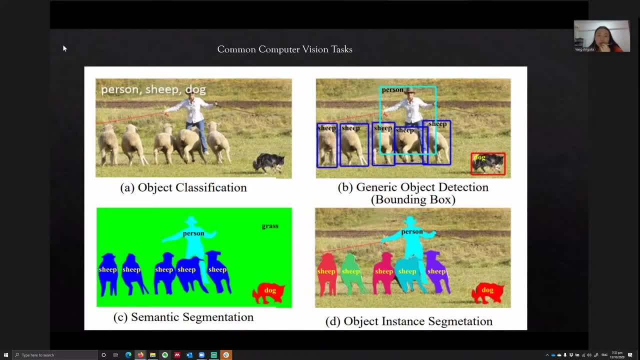 object classification. object classification, basically, is the full question. i only need to ask whether my target is in or not in this image classification. so among all these tasks, uh, it will be considered as a relative low level task and one step more. i i'd like to know. 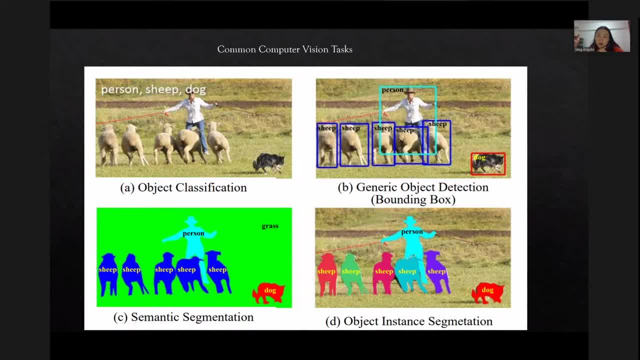 like, uh, beyond whether it exists or not, i want to know, uh, where is location of my target on my target class or my target instance? so that comes to the definition of generic object detection and beyond that, i'm not just satisfied with the location and the existence, but 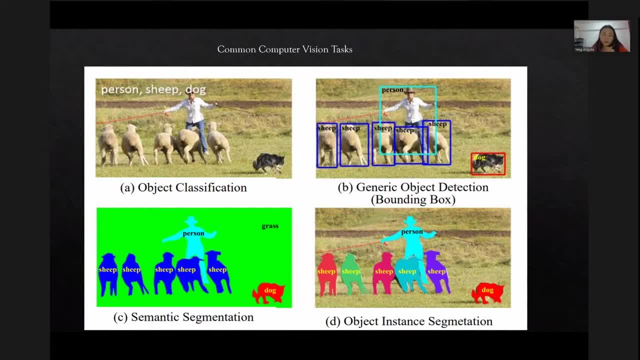 uh, i also need you to control the specific instance or specific class into in these images, in this inputting data. so that's how the semantic segmentation and the instant segmentation comes out. so for semantic segmentation, i only need to control the same category like all the entire classe. i need to include data inside the base. 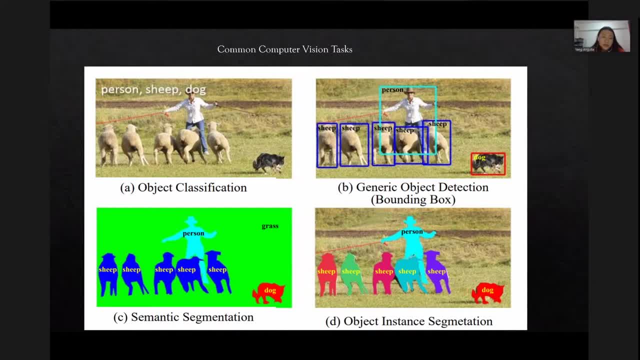 these five shapes are all in one color because they are in same shape category, but, for instance, segmentation, which is a more detailed task and also high level understanding, i need the neural networks or the algorithm deep learning models to help me contour each object and their corresponding class category. okay, so this is basically the um definition of 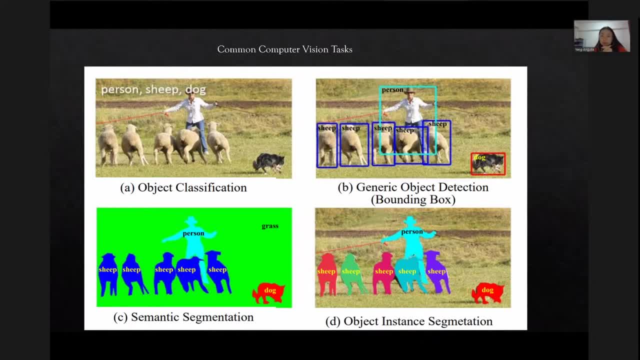 of these, um, these essential tasks, then we will go go through one by one, from the classification to the object detection and then to the semantic segmentation. see how uh does this uh classification, classic computer vision task evolve and what new elements was added in each stage they evolve. 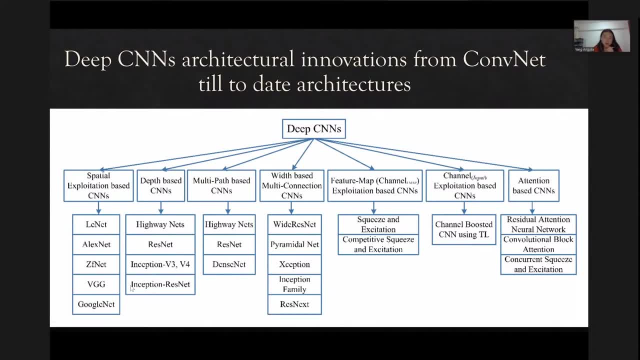 so yeah, first thing first, because this is the most basic one as the, it's the basic one as the um classification task. so, then, what we're going to do is we're going to follow the like, the one back in the first phase, and even a floodplain um the first sake бол腸. 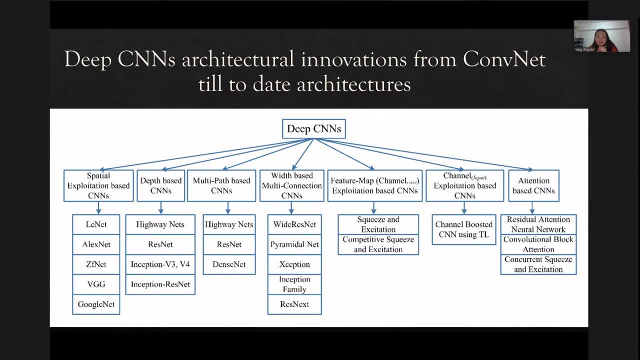 process History, one like one page back, and i just wrote the sieve. i mean, like you know, in more, a lot of awhile, as you're enthusiastically looking, i'll show you right, yeah, then you just can. just昨 afternoon, you just you, um, since this is the story, then the uh week. okay, let's go see the next one. 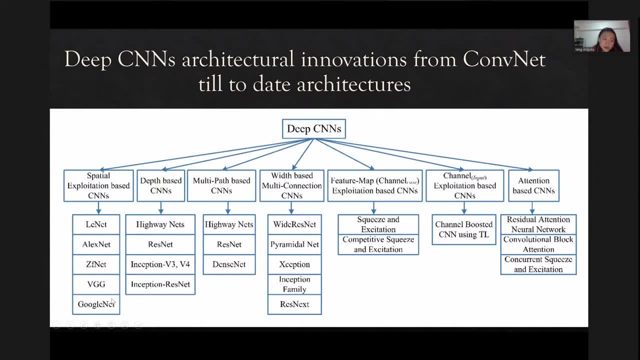 okay, so this is the the type of information that the um job of the early date school details on. uh, we can see there are several kind of Indo codenames there here still are, but you can see one in each one, which um is usually called the knowledge of deepbeits. most of these editors work in a uży yuppie movements category based on ideas you cangasp. 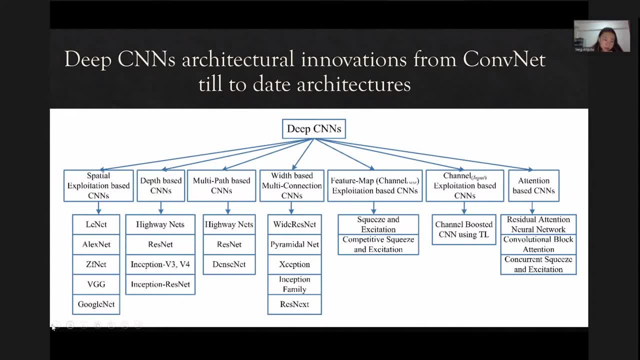 net, Alex net, VGG and Google net, which is also the Inception net version one, And in the rather early stage, depth and breath makes the same and more powerful in performance. So then we will have the accordingly Inception v3, v4.. 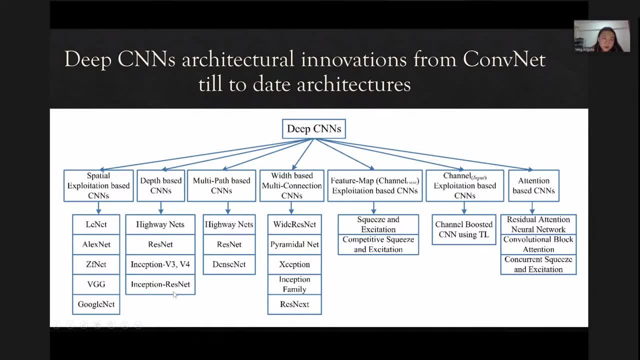 And they're basically like: the deeper, the better categories. So we have the rest net and also the combination between these two. then there are, there are there's the multi pass based asians, And here we have the. we have the clever connections between all com layers. So the rest net and 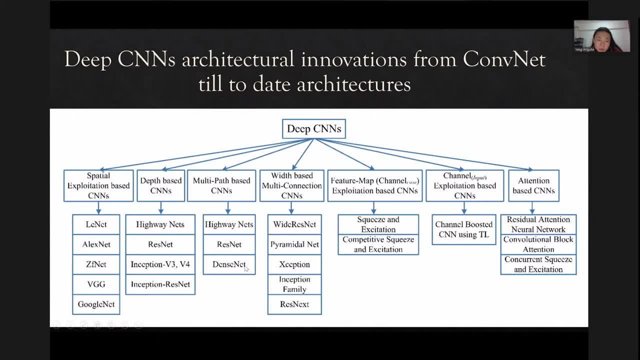 the dense net come out and which also be another milestone. Then another one is the width based multi connection CNN, which also this one's the pyramid net exception and the rest next, which is also the changing format from the previous classic models and for also for 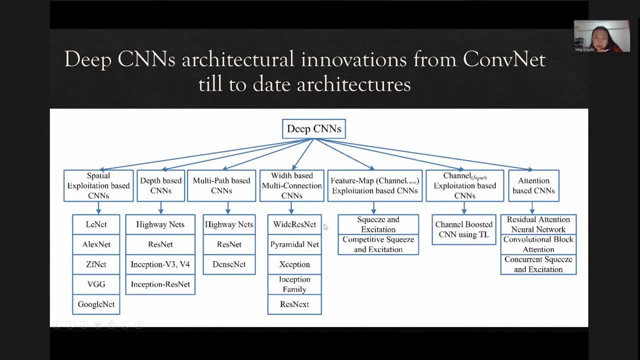 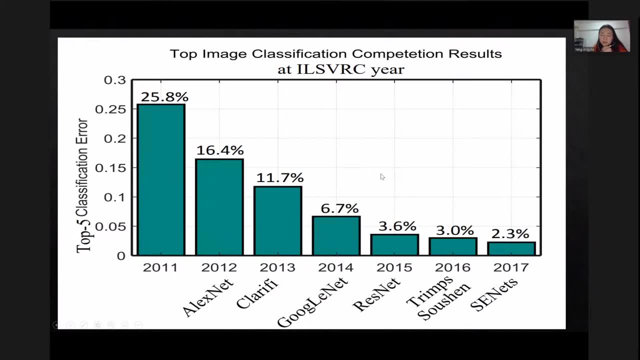 the other three categories. So these are categories basically based on their characteristics. we can also see from this, from this perform performance results, which also can explain how the, how the classification model evolve according to according from the 2011 to 2017.. So for for 2012,. 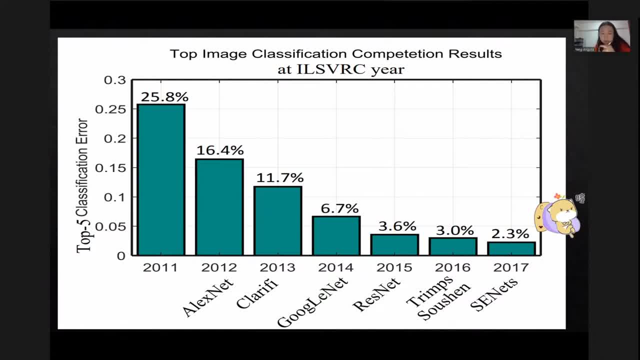 the Alex net came out, which is, firstly, use the GPUs and firstly reach the very promising performance to beat all the other handcrafted based models. And then the, the deep, deeper net, the Google net, rest net, sort of VGG, come out. and then 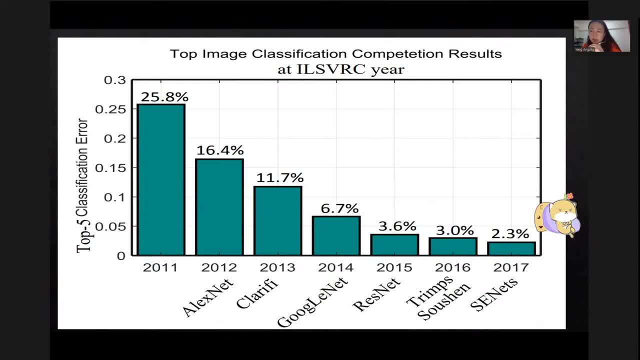 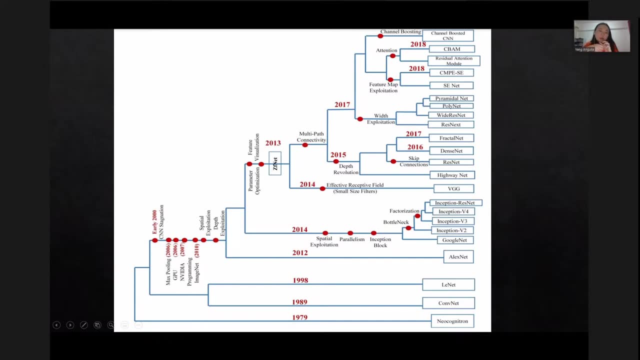 can decrease the top five classification arrow into as low as 2.3%. So So we could take a closer look And then we could further take a closer look according to the time, As long as- as early as, like I said, to the 90s- we have the net and we have the very initial count net in this. 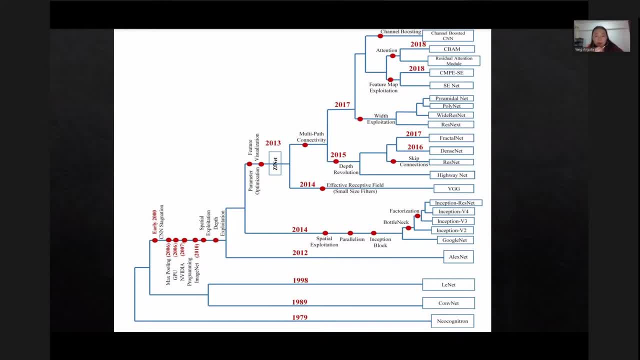 computer vision community. Then then 2012,. we have Alex net. In Alex net, it could be treated as a groundbreaking model which, firstly, utilize the GPU and the first, utilize the multi layer networks And also, like the, the three factors, the data was prepared for the large competition. 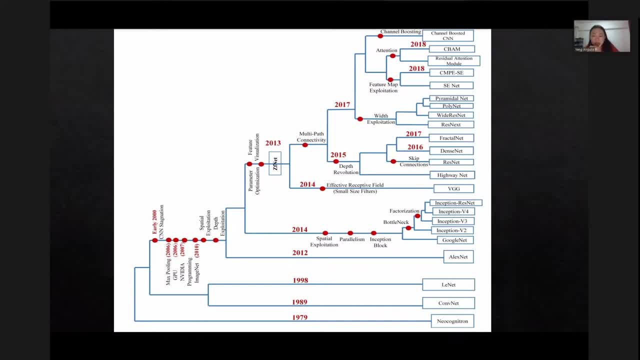 Then, and the GPU was set up that time, And also deep learning was the first time show its power in this image competition. And then in 2014,, we can see this time the exception family, so called a Google map, Google net family- comes out and the take. 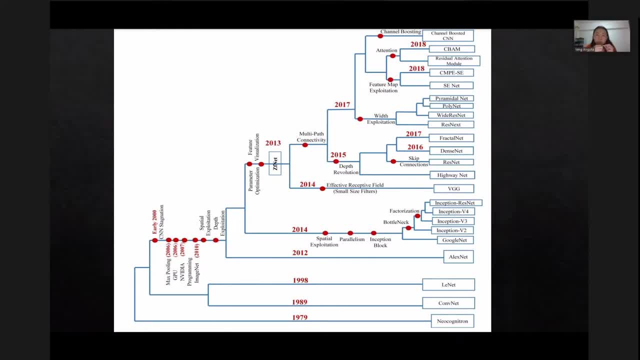 the dominance. Then later we had the. We have for the better parameter optimization. we have VGG and we also have the ResNet and DenseNet, based on their specific layer connection design and also with skip connections. we have ResNet. 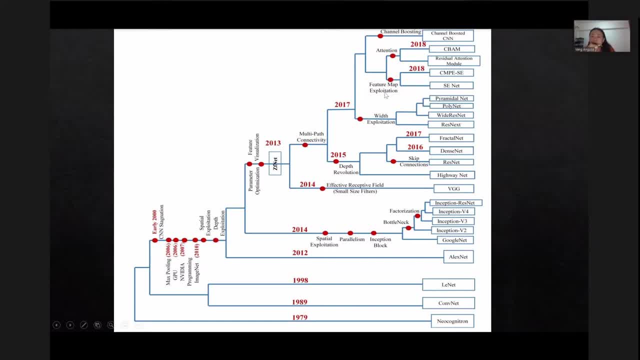 And later during 2016,. we have PyramidNet, which explores the widths in the convolutional networks, and since then we have one more milestone, SCNet, which further explores the feature map, And later the attention mechanism was also involved in this convolutional architecture designing and till 2018, basically, we could see there's almost the end of the architecture, innovation, exploration. 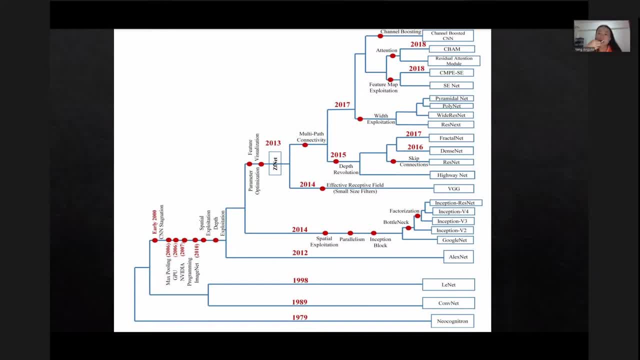 Because till now we can have very very least effort to train a network to apply our image classification. but in 2012 to 2014, these two years, there are many new ideas about the different convolution design or network design comes out. 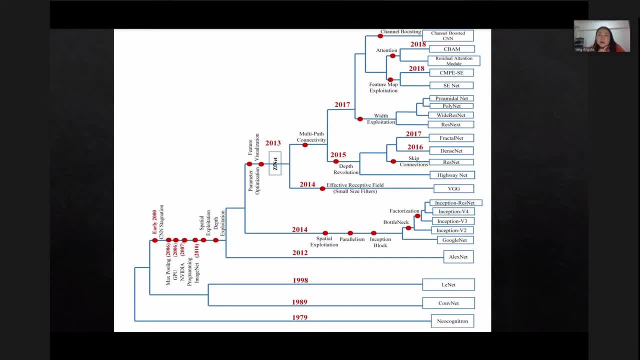 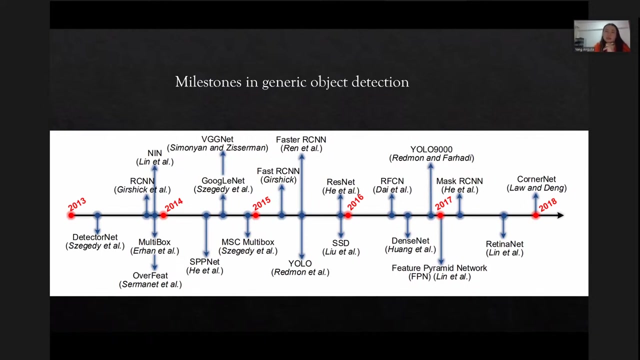 And yeah, so basically now the image classifications also was considered as a very basic and mainstream application in the industry. Okay, so with the basis of the deep learning complex And also the deep classification comes out, the traditional object detection task also got evolved quickly in these years. 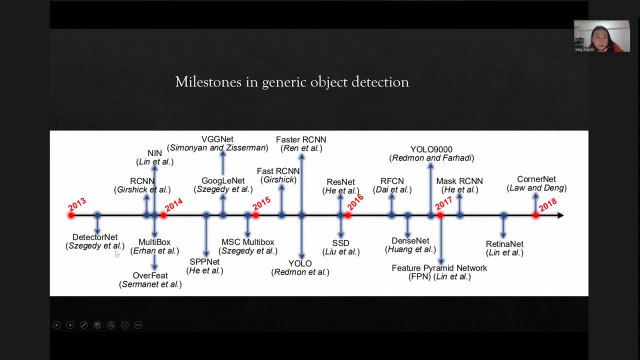 We could see like before 2013,. there's no such Deep based detector comes out and after the AlexNet and DetectorNet we come out. our famous RCN- the first RCN- comes out to apply for this object detection. 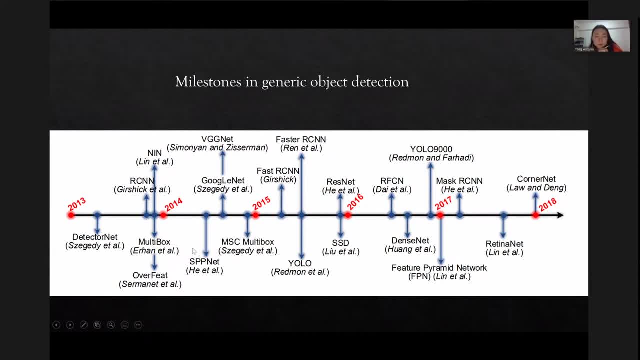 Then the SPPNet, which used the spatial features, Then the SPPNet, which used the spatial features of the pyramid network architecture also comes out to better understand the different scale of the features. Then was the RCN family takes the dominance. 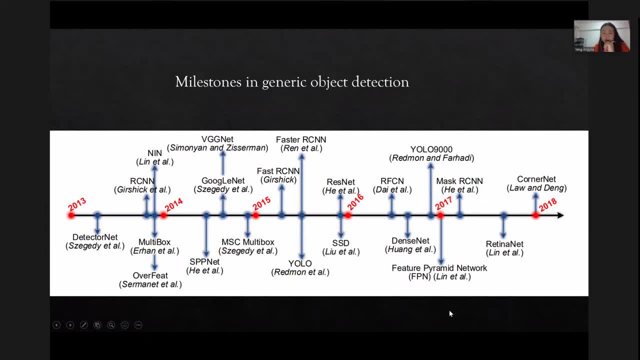 And since the RCN families have a sort of problem in the efficiency more advanced, And since the RCN families have a sort of problem in the efficiency more advanced, And since the RCN families have a sort of problem in the efficiency more advanced, 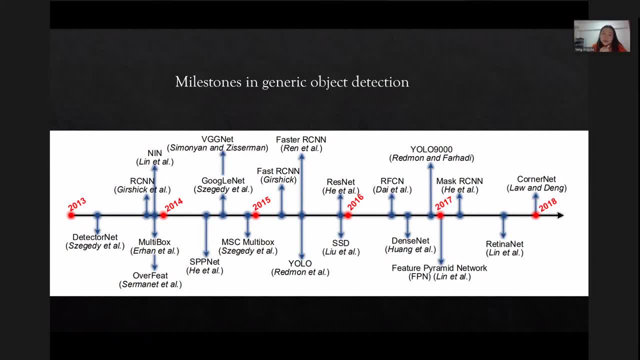 we say one stage detector such as ULO and SSD was also being proposed And being now, which is also widely used in the industry. these two models, And later there's also mask RCN, which can also both can, And later there's also mask RCN, which can also both can. 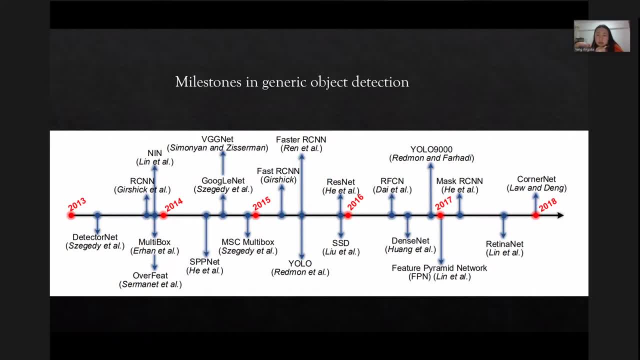 both deal with the image segmentation and also the image detection at the same time, And we could see also like they keep basically the same pace with the image classification. So till 2018, they sort of converge to a. So till 2018, they sort of converge to a. 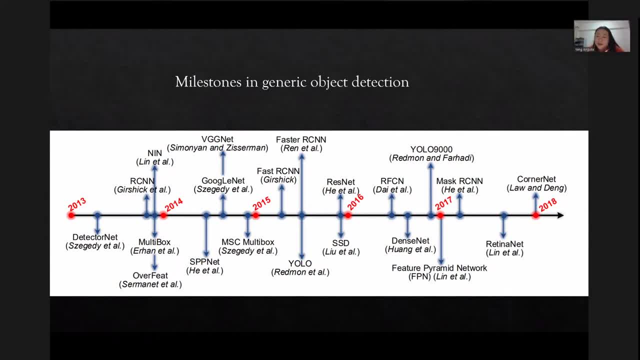 So till 2018, they sort of converge to a, they converge to a very mature state And basically this is the current object detection environment. And basically this is the current object detection environment. But still, yeah, there's multiple new new methods coming out. 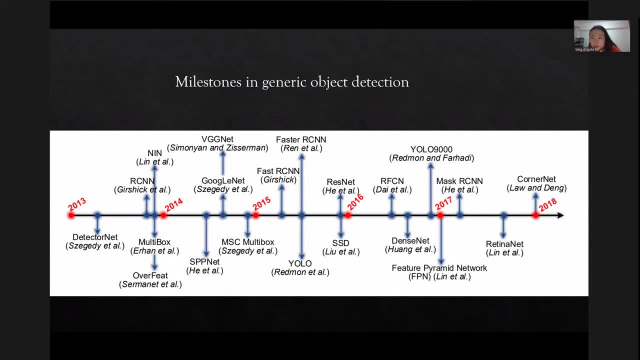 which was more fine tuning, and also some advanced technology integration into all this integration, which was more fine tuning, and also some advanced technology integration into all this integration. But still, yeah, there's multiple new new methods coming out, which was more fine tuning, and also some advanced technology integration into all this integration. 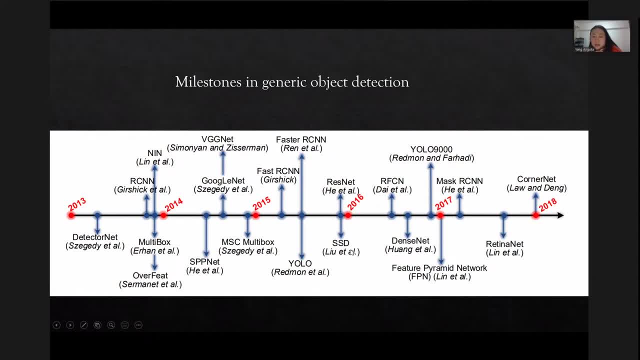 But still, yeah, there's multiple new new methods coming out, which was more fine tuning and also some advanced technology integration into all this integration. But still, yeah, there's multiple new new methods coming out, which was more fine tuning and also some advanced technology integration into all this integration. 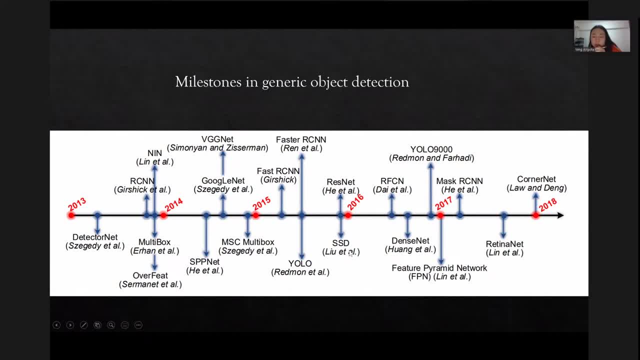 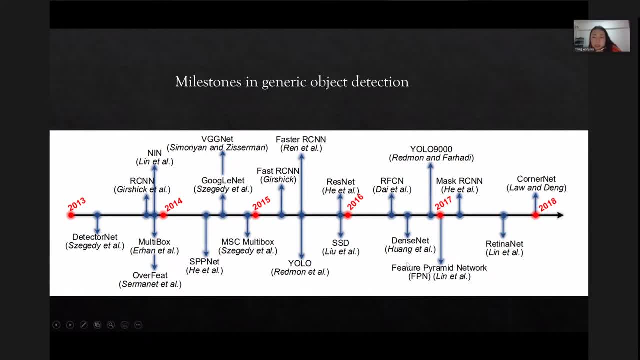 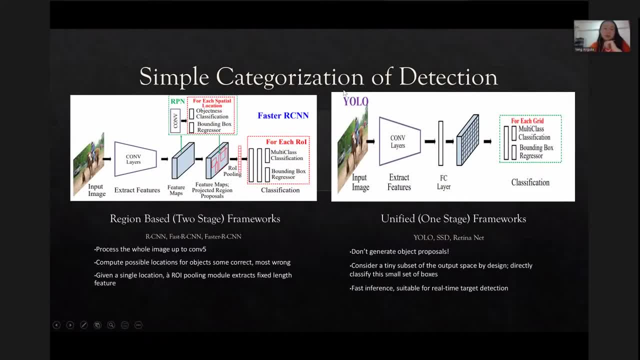 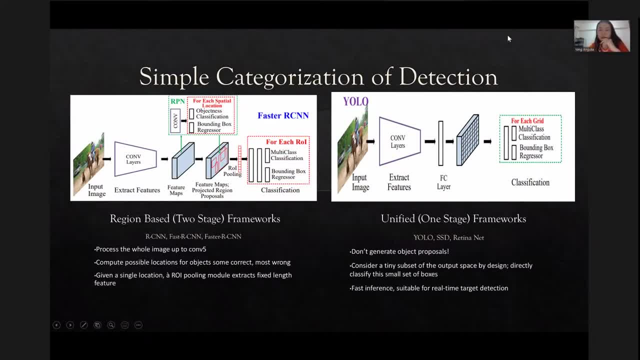 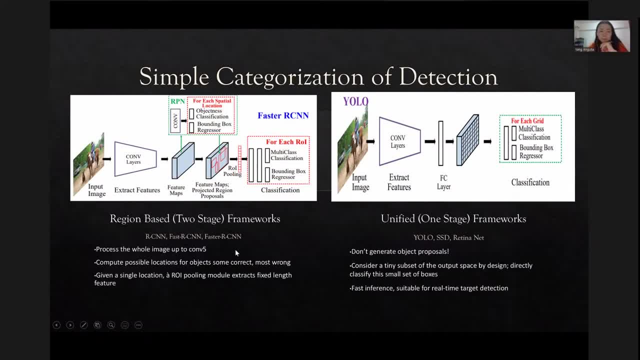 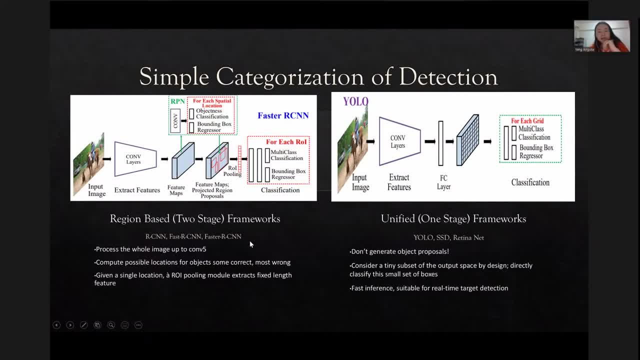 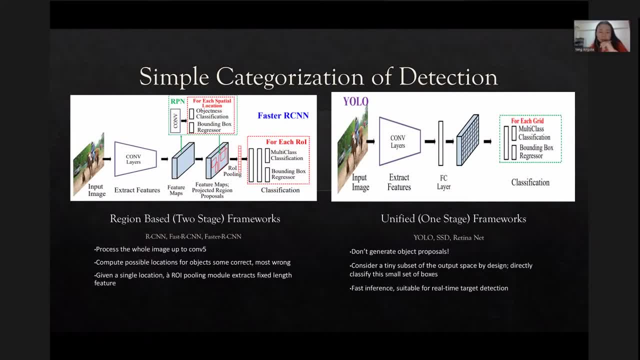 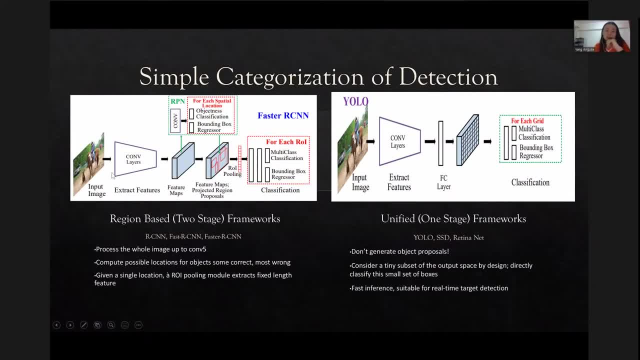 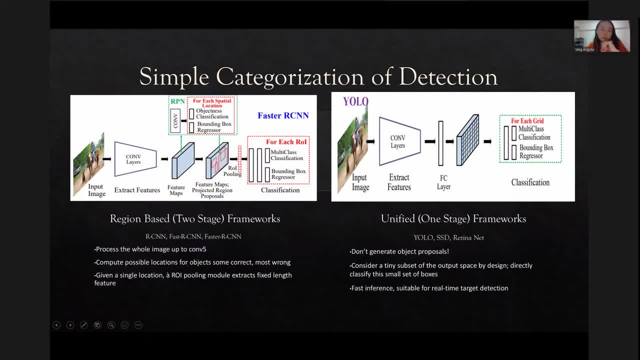 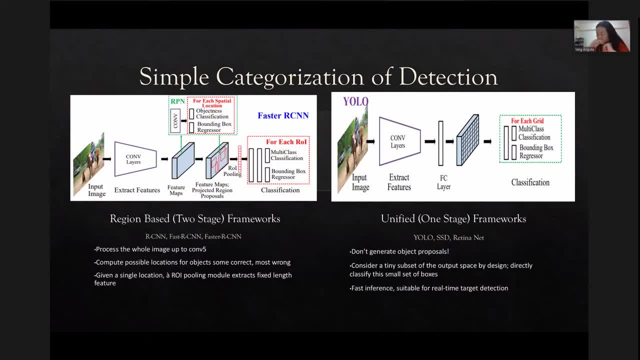 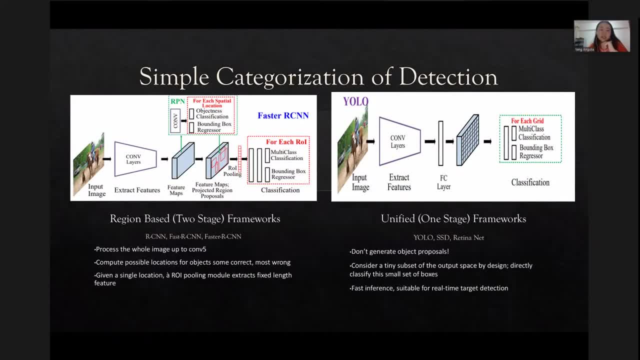 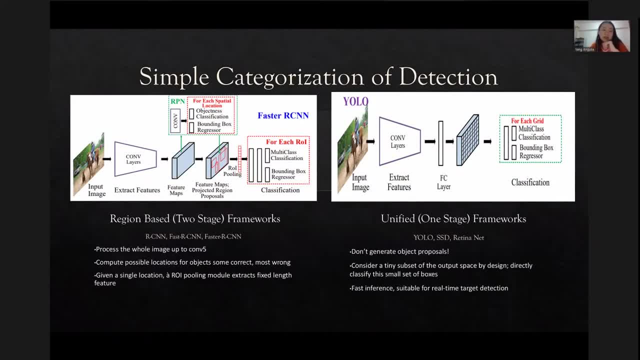 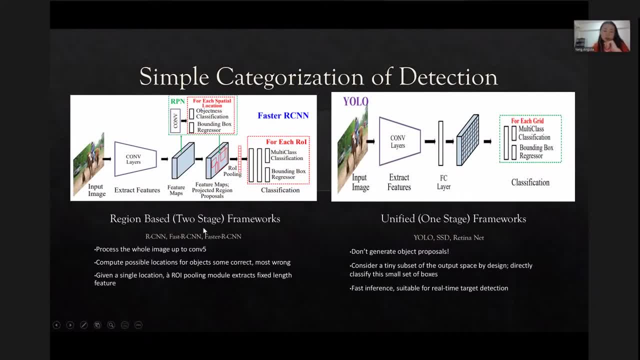 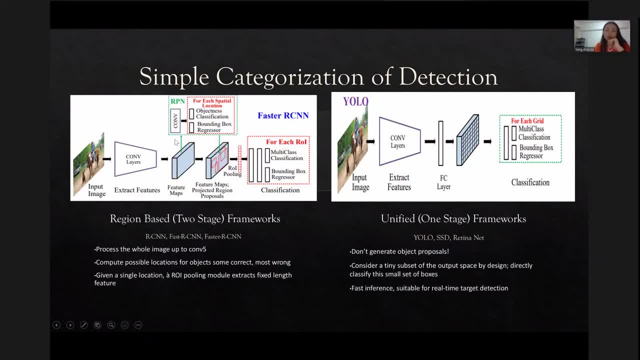 which was more fine tuning, and also some advanced technology integration into all this integration. But still, yeah, there's multiple new new methods coming out. feature is there will be a proposal extraction stage for extract multiple for extract the multiple bounding box. 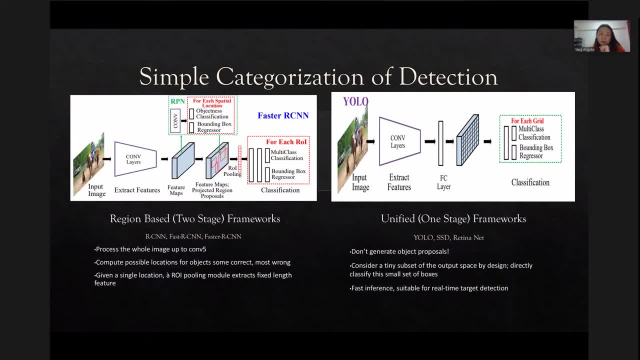 And then we regress the final answer and also do the classification for each region of interest. So this one is also highly increased the performance, but somehow it was time consuming and we could see the two stages not very, very efficient. So that's why the YOLO and the SSD. 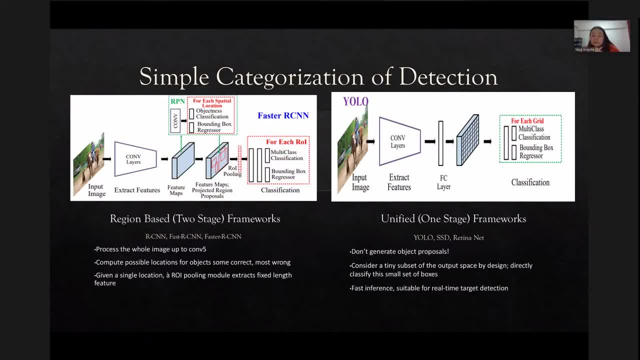 those, the representative of one stage frameworks, comes out, So they do not require generate object proposals. So they consider only a tiny subset of the output space And they directly go one pass to classify the small set of the bounding box of our potential. 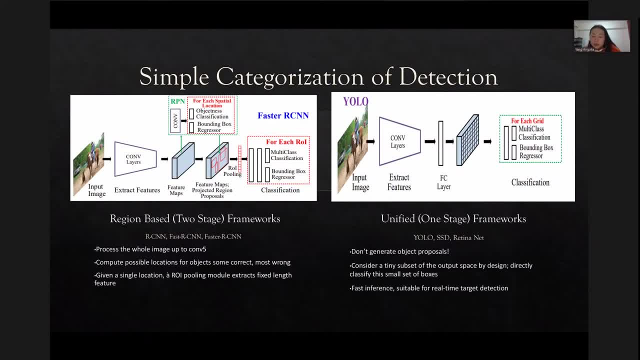 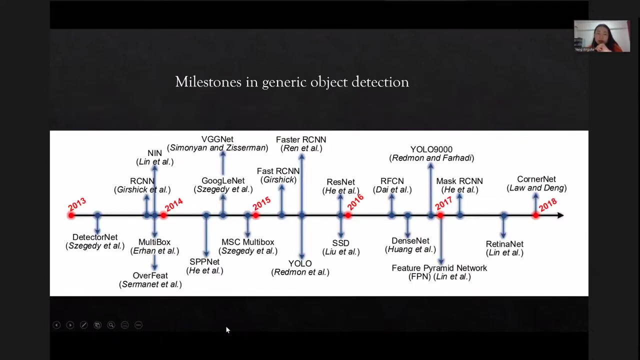 the potential predictions. Yeah, So it can basically reach faster inference and which is also suitable for the real time target detection. So this is basically the growing of the detection We could see. basically the detection also keeps the same space with image classification, with groundbreaking the representatives. 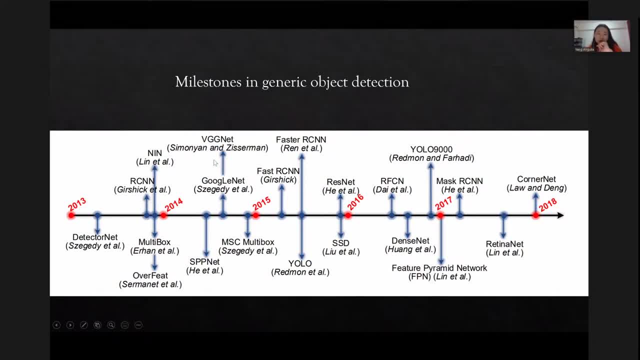 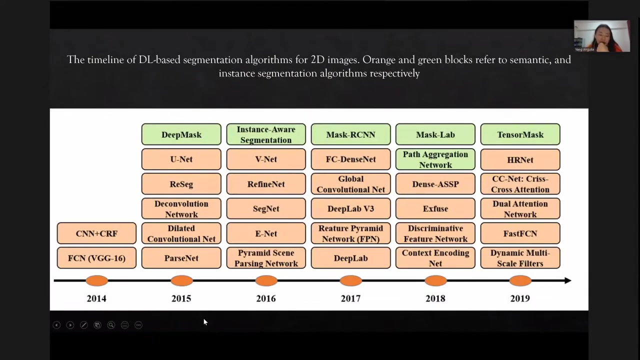 the target detection models has been proposed, like the RCNN series and the YOLO series. now, the modification and also the updates are basically inherited from these established what we call traditional models. And the last one I like to briefly mention is for the segmentation. for 2D images. Segmentation is also considered a high-level image understanding. 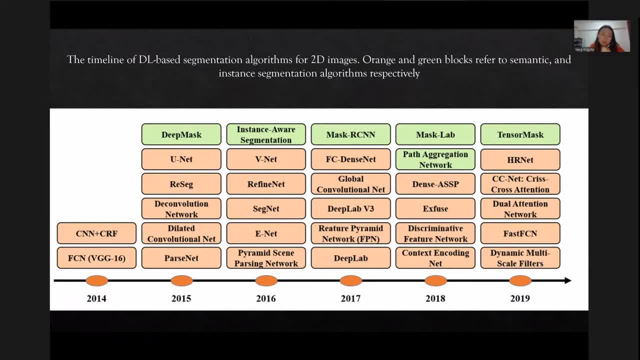 task which now has been widely used in the autonomous driving and also medical image analysis. So we could see, in 2014,, the very first fully connected network, which is also very well known, comes out. then it's some of its variation continues and also the very special U-Net. 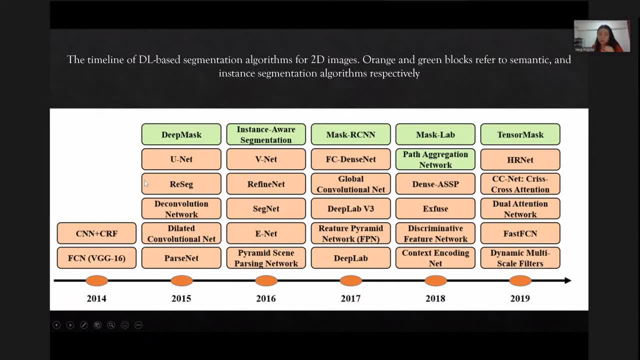 and the V-Net comes out For basically the medical images analysis and, during this period, the, the pyramid, because the the pyramid networks also are involved- into a better the in in the performance improving stage and then mask RCN and deep lab, v3, these, these, so we are like also well known and 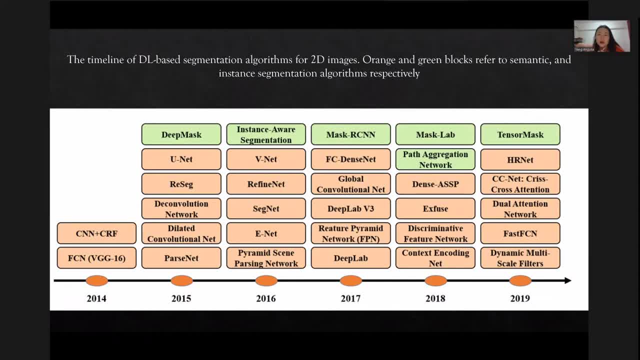 now commonly used, the model are also come out, and then there are some more like past aggregation network and the, the hr net, and also later the attention was also was introduced and the dual attention network comes out and for now, like the deep lab, is also being widely used for the. 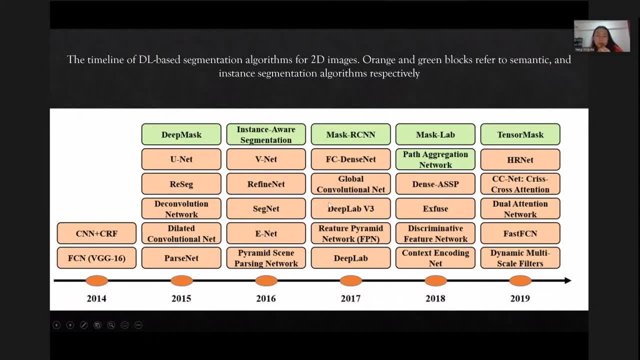 as the, maybe as the backbone, or maybe as the final model in the real world use, or maybe in the, in the, in the research papers, and you can see there's always there's also a converged process from the very first brand, a groundbreaking work uh, from fcn to uh the current, like the rather mature, deep. 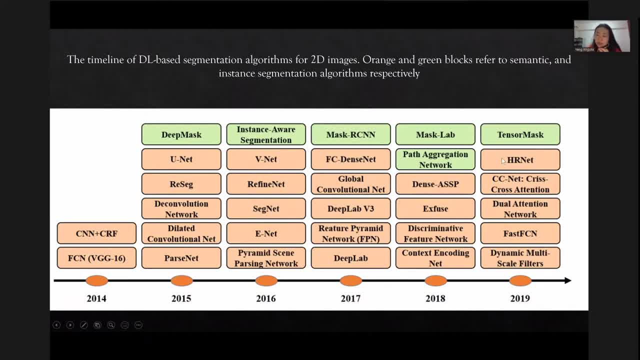 deep lab v3 and also like uh attention network or hr net. so um these are the three uh very essential and very basic tasks of the computer vision we could see. there's uh um expulsional increase or very uh quick changing period, basically focusing on the uh 2014, tier 2018 and during that time period, many 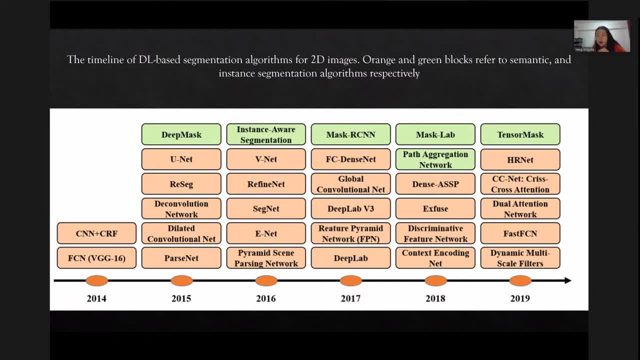 classic methods like our currently used resnet, inception net and the faster rcn yolo, and also here like mask, asin and the deep lab, has been wildly used and during this period they come out during this period, and for now we'll see for this uh. 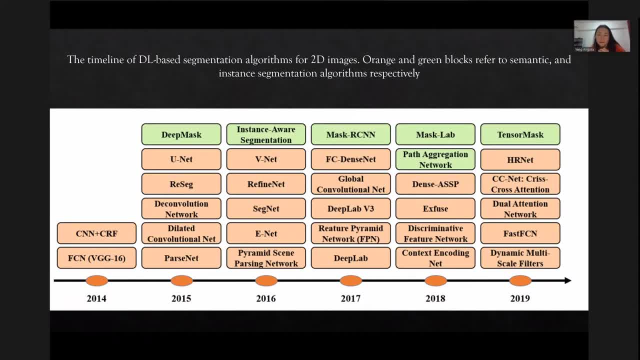 from scratch. i say like from scratch methods. reconstruction for this basic task, which currently is, is few, because now for for all the existing data sets and for these tasks, these uh, these models now can cap, like uh, most of the efficiency problem and also about the performance, about their accuracy. so 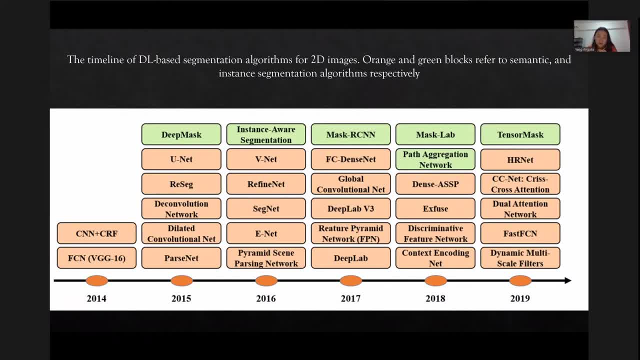 uh we could see for for those. if you're, if you are very interested in how to make your your like, make your idea combine with deep learning, combine with deep computer vision and make into product, try to commercialize uh your business with the help of uh deep cnn, and i'll suggest like for: 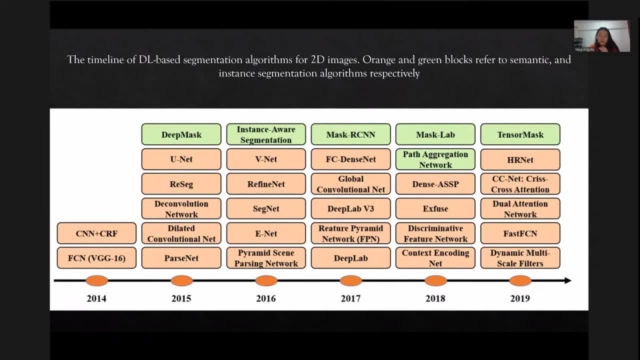 this mature model and, uh, for they might be the best choice for you to give a first try, because these traditional models now, after two to three years, they raised a very large community to contribute and to deploy in different devices, like in mobile, like in the mobile phone or in FPGA, or in the web serving. so 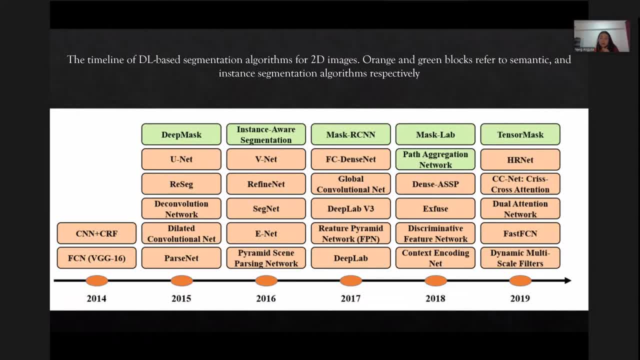 the, these tasks and these models are the mature and ready to industry for, for for this current stage and but but for the like research exploration and for the further, like the architecture exploration, I'll say there's maybe relative limited space for this task. recall, like our three factors, because 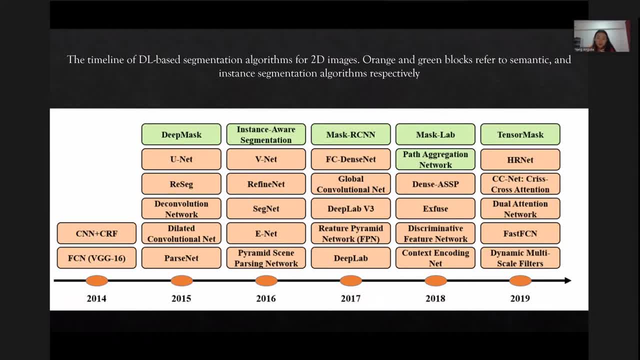 the new coming public data sets is also follow a curve, almost like these three tasks here: 2018 or 2019. basically, there are no much more public data sets comes out and for the existing benchmarks those models can handle very well. so if you are try to start with business or start with 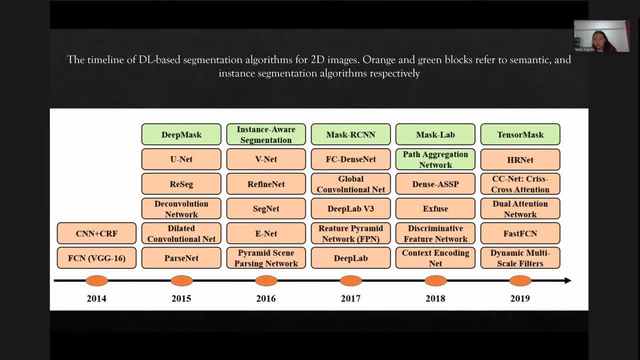 application. I would suggest maybe you can start with those traditional or classic classic model first and to give a shot with your first, first try and application. and for those who are willing to, very willing to see what will comes next, this is basically personal my opinion, from my 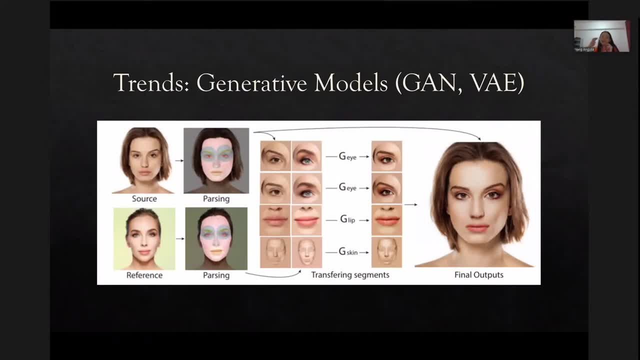 this is basically personal, my opinion from my. this is basically personal my opinion from my Civil engineering course. so for the third and last, I so a big, big, like most such big loan, like daily paper rating or daily reporting, like daily paper reading or daily reporting. 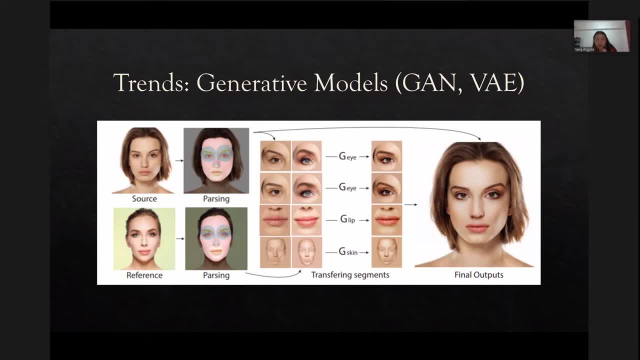 like from, from from these years, a report and also the conference proceedings, Our, Our, I am going to briefly share with you, briefly share with you. So one trends will be the generative models we also see the Kellan and the Veo doing. basically they are two different architecture, diaphragm, types of network architecture and customer两wers embedded Norway, that specific being not to be used, accordance here, hardwareère, Disco naturals and websites without sleeps, pair pick up software to to the 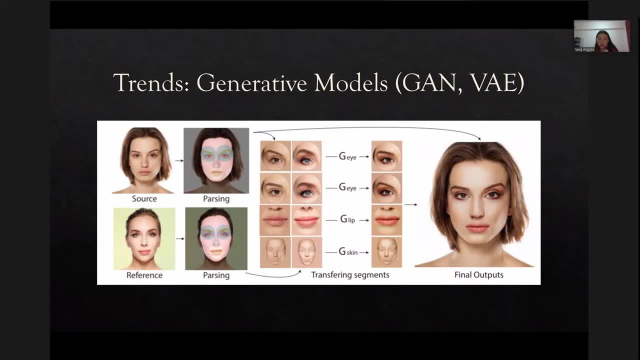 Must Employ, Must, Employ, the must, employees types of network architecture, but they're doing the same thing. that's uh gen generate the, uh, the very real, realistic, uh the pictures. so uh, this one currently has been widely applied posting application. but application will say more like it's entertainment, like recently. 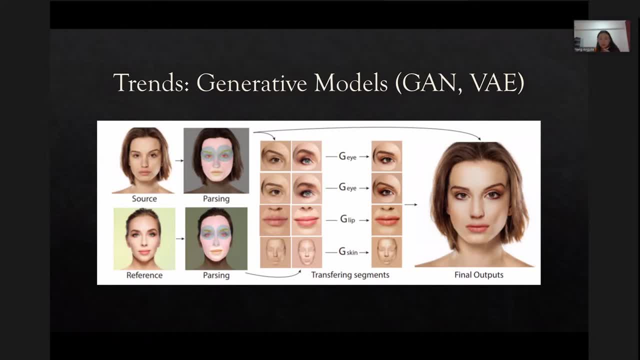 you can generate a makeup based on your original input, or maybe you can style transfer other ones, the the face, or you can style transfer the monet or then go their their paintings, the style, to create some, uh, our artistic uh pieces. so, uh, this one, but this one still uh, currently remain large space. 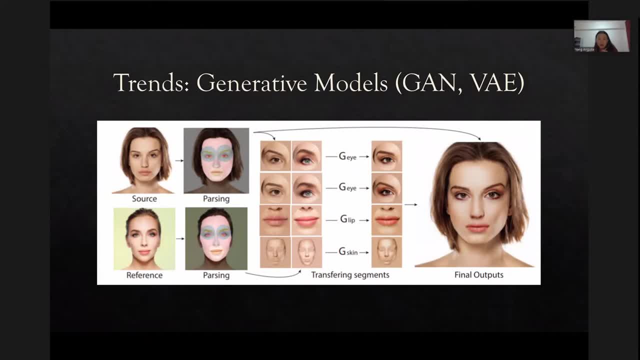 in the, in the research. in the research because because current the generative model training is very unstable and which is also resource consuming. so this would be a great direction to explore and if you want to try how you can generate a different look or or even non-exist uh pictures, maybe you can try with the existing uh. 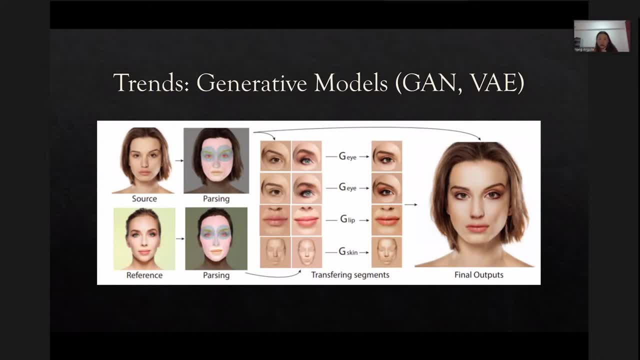 existing gen networks. i recommended you to to check out with uh. some works out from the nvidia ai. they developed a sort of style again and some very high resolution generative models to generate the high resolution sharing the, the model you're using- human face pictures- and this one should be very interesting and also can be applied in sort of 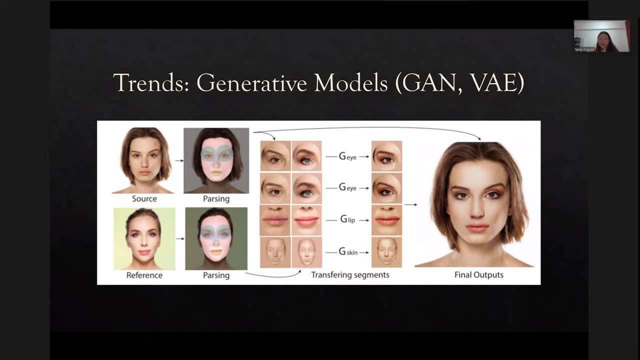 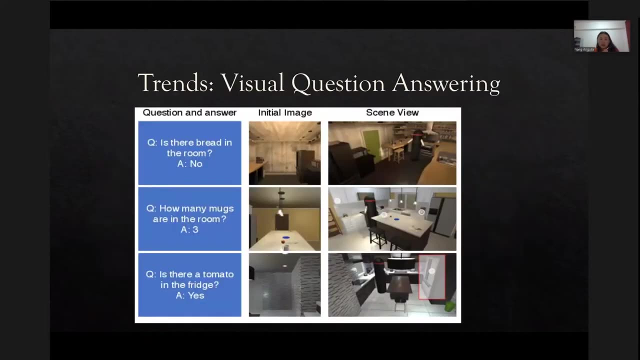 entertainment, entertainment application or networks, like the face swap application, sort of things, and also, like previously very well known, the deep fake. yeah, and another trend is vision combining language and natural language processing. um, because for for now, i mean basically folks uh, basically due, uh, on the 2d images, which is the rgb image, 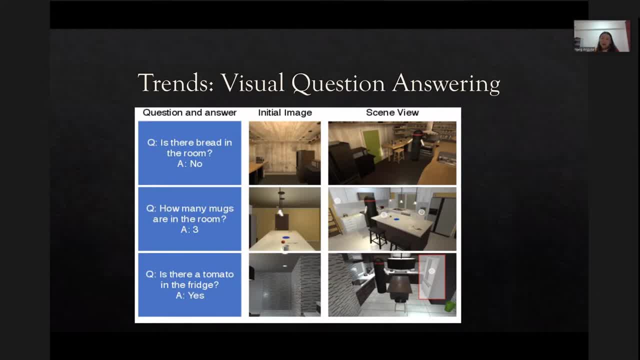 is: uh, we are basically focusing on um, their grid-like matrix in like in in the network or in the computer system. so but but for the language they are not that structured as image can be. so there's still a lot of the difficult dilemmas and problems. 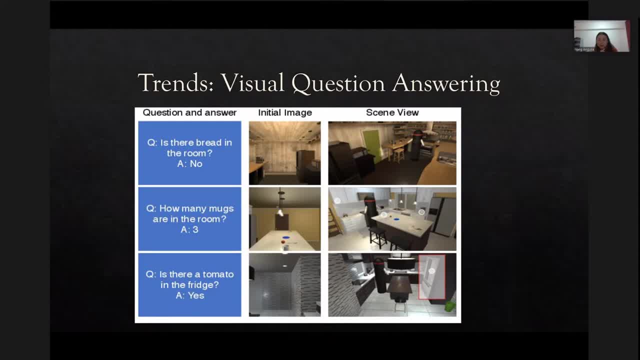 um, but but for the language they are not that structured as image can be, still exist in natural language processing. so this one would be a very interesting perspective to try to combine the language processing with the image to give a high level understanding. so because for people we are not just looking, we are also hearing and maybe we're 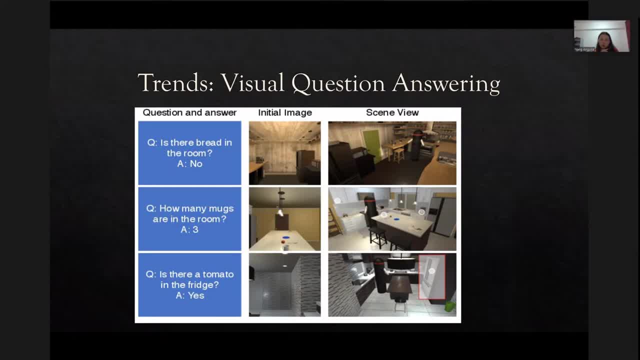 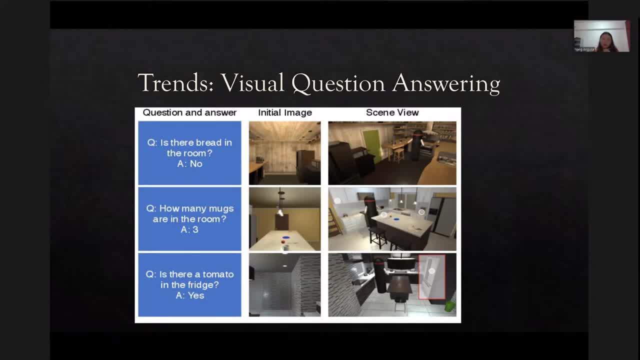 uh video and also the��상 exam- that with the research of these visual question answering, which is also like the the language and images task combination. this one is not very, very massive, very, very mature or class classic models like uh, object detection, object segmentation, so this one can also be a very potential way to uh. 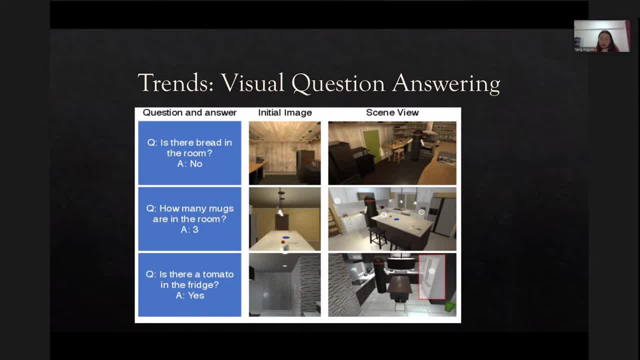 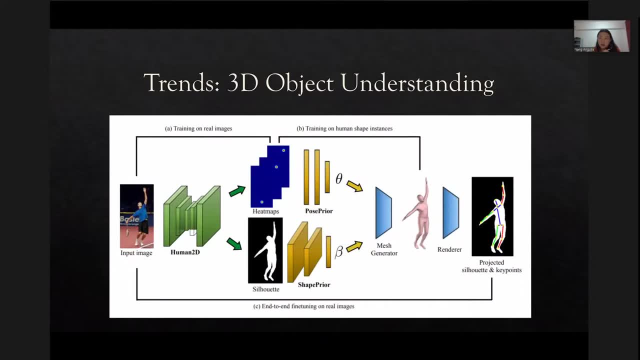 control of financing fields, in other words, your research or your application. And one another thing is also the comes out in recent two years, which is the 3D object understanding. Also the understanding maybe including, like the pose, estimation and the segmentation or tracking or the action recognition sort of things. 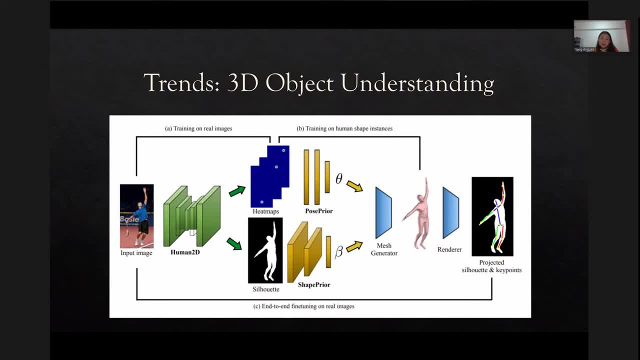 So also this one should, thanks to the availability of the 3D dataset, comes out, because previously for the 2D images, one difficult part is that we cannot see the overview of our target images, especially in the task of the person dominated, like in the person re-identification. 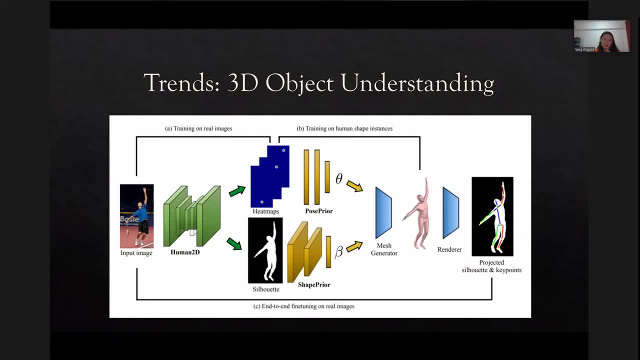 we need to access the front view, the side view of the same person that we can verify his identity. and misidentification also always happened in this hard occasion. So when the 3D data is come out or the 3D reconstruction is enabled, this problem actually can be solved rather easily. 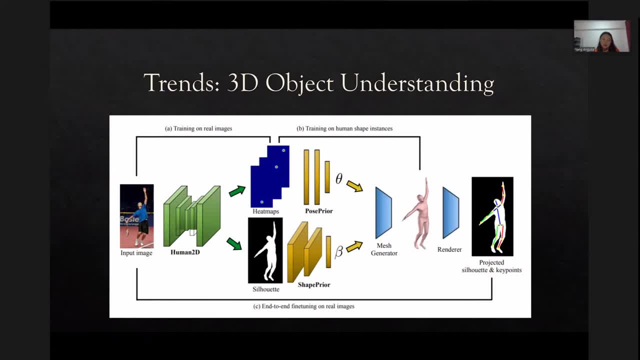 and which is used to be very difficult In the 2D dimension, And that's why I think this is also a good sub direction to explore. And I- okay, I think it's now one hour already, So okay, Okay, Thank you. 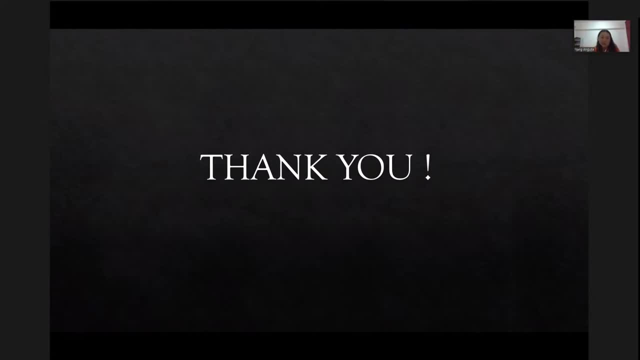 Thank you everyone for joining me today And later in the question answering session. maybe we can discuss more about my personal sharing And if you've got any questions, or Yeah, we have a couple of questions. Ugaliya, Okay, so, or Jason is asking for Q&A. in your opinion, 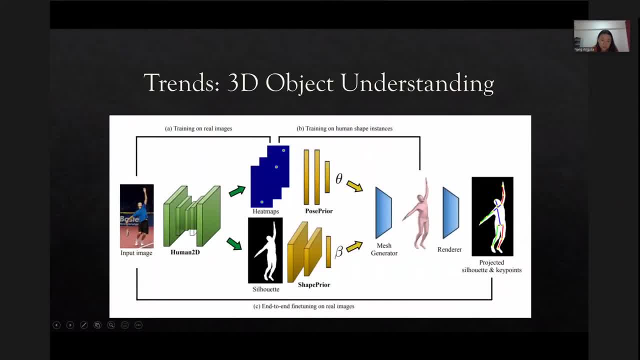 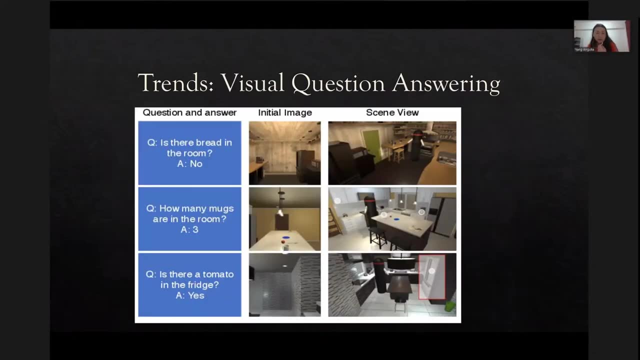 How, for you know I skinny now. where have you been doing this for species? you know enthusiasts for people who are just starting out. how can they get involved into developing their own code for computer vision applications, or is it just limited to published algorithms? so, uh, due to this uh visual question answering uh task, i'm sorry i i maybe missed. 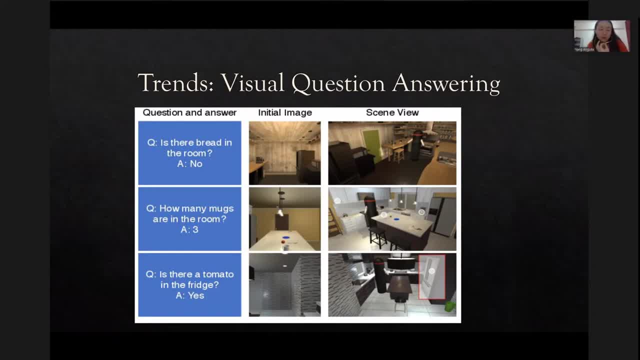 like jason, is asking that you know how, if someone wants to uh develop their own cv application, how can they start off? from where can they start? how can, how can start a cv application, right, okay, so for start, uh, i suggest maybe uh, because for for the basic, 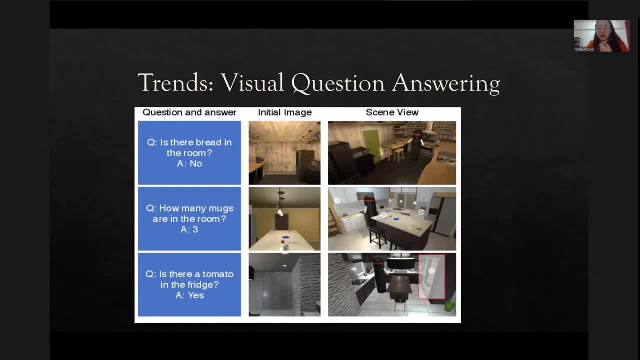 uh, basic advice will suggest you to try out, uh, amnesty, a digit recognition tutorials, sort of things. but i say, maybe you can pick a specific task you are extremely interested. um, and then i think github can, can help you to find a uh, very high star like repository. 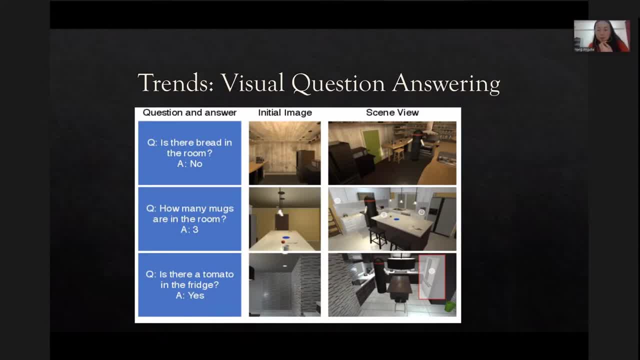 or some example project, and i think you can refer to their implementation and then try to update on your site. and also like read their code first and do the multiplication based on what you would like to change and see the effects when you change sort of like parameters or layers and 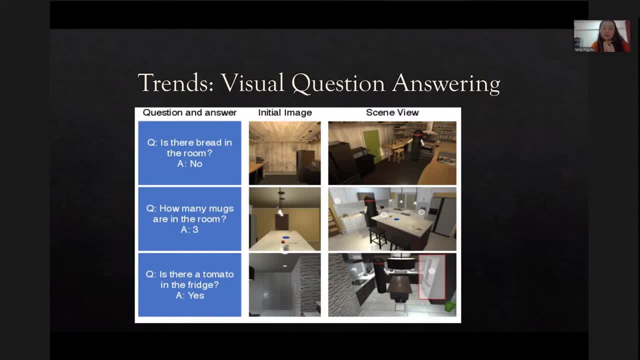 that this maybe can help you to firstly understand the specific task you want to dig in. Yeah, this is All right. all right, I hope, Jason, that answers your question. And again, another question from Jason is if you wanted to build a system. 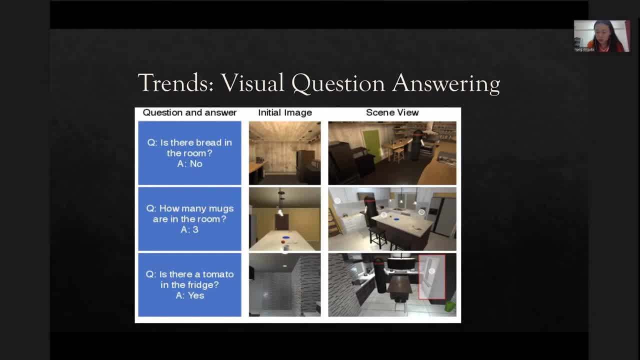 which recognizes actions in a sequence, like some actions in a sequence performed in a sequence. what kind of algorithm would you suggest? Oh so, for the action recognition, accurate recognition, I recommend, like there are two models I remember called I3D and C3D. 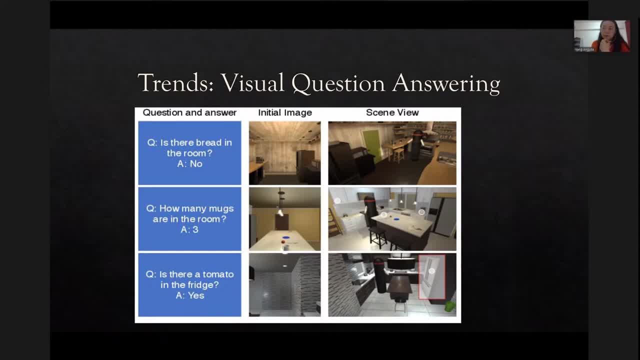 These are the basically also a well-known algorithm developed and deep learning based. These two models maybe can help you, And which is this is basically due to the action recognition in the video sequence. Yeah, I think you can refer to these two existing methods. 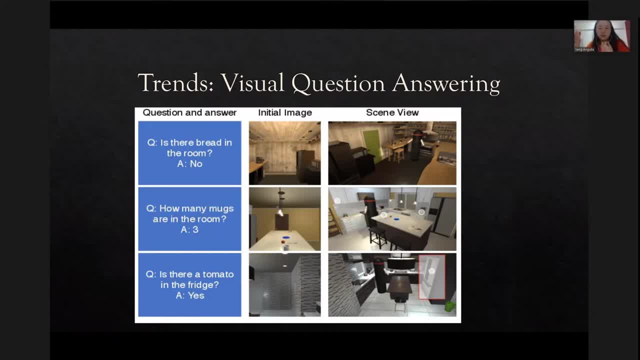 and check it out first, Then maybe, if you have another idea, you can develop on your own. Yeah, All right, all right. And another question, a small one, is that you know, I think in your slide deck there was something where it could translate a word. 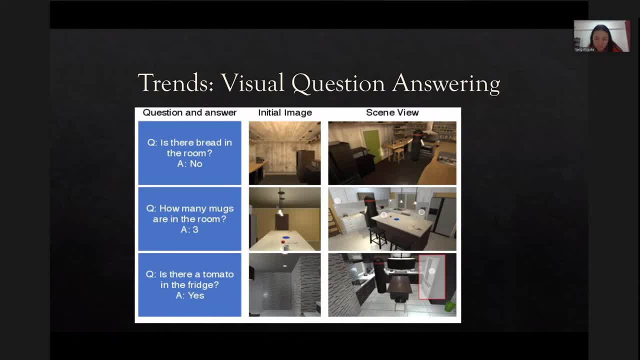 when you click on that. So people are asking: what was that application you are using that can translate a word in an image? Translate what in an image? The app- Yeah, For that. I think they saw that in your presentation, in your slide deck. 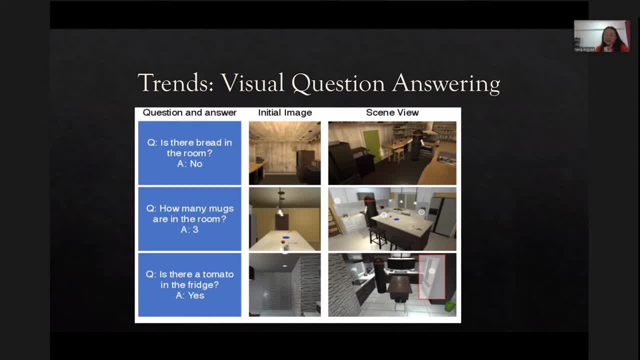 Oh, that was my translating app, which is a wrongly Okay, okay, okay, all right, Okay. so that's it, And if I mean you know, know, uh, people who have your any questions, any further questions, they'll reach out to you on. 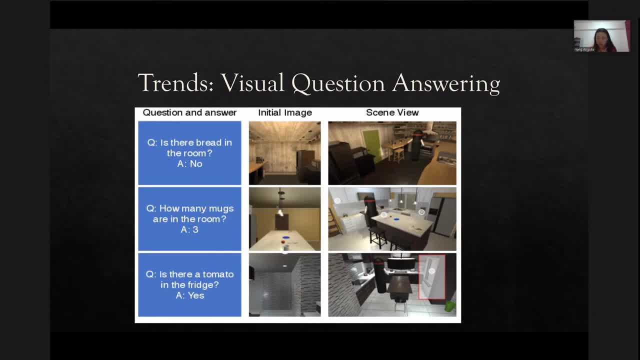 your linkedin if they have more questions or more insights to discuss with you. and thank you for the session. angulia, thank you for spending time with us. thank you for this absolutely wonderful deep dive into computer vision. uh, so i i kind of like the 3d. uh, you know, action rendering model was very 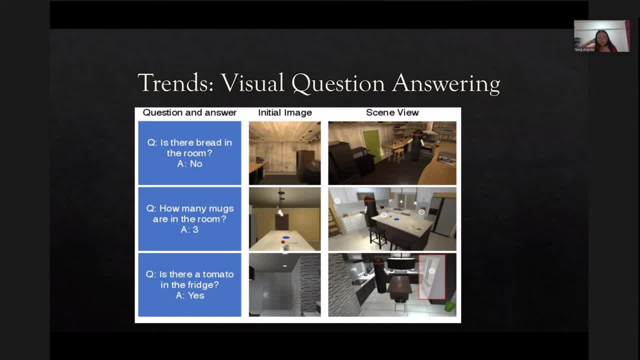 interesting and thank you so much. we look forward to having you again. in case you know, you have more interesting things to share with us, sure, sure, thank you, priyanka. thank you for inviting me. no problem, a pleasure to host you. uh have a, have a good day and uh stay safe. okay, thank you, thank. 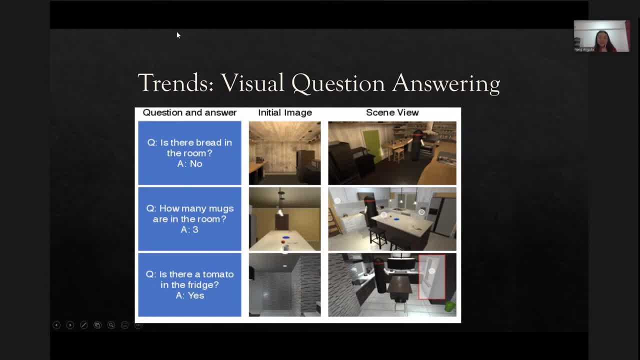 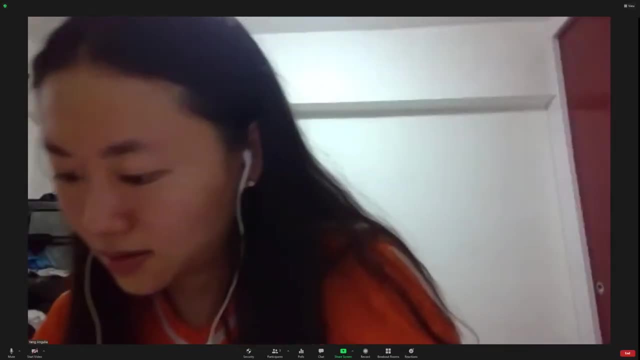 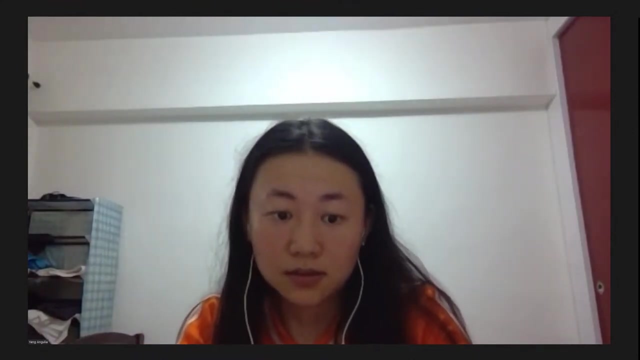 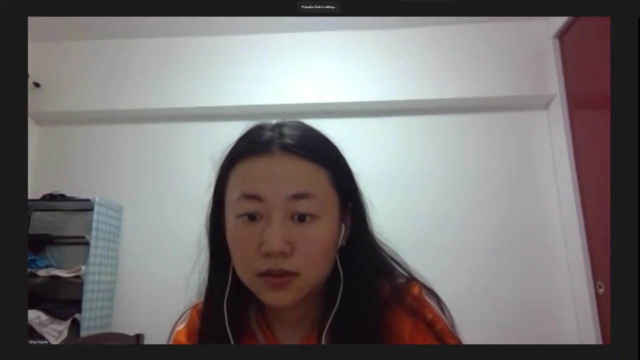 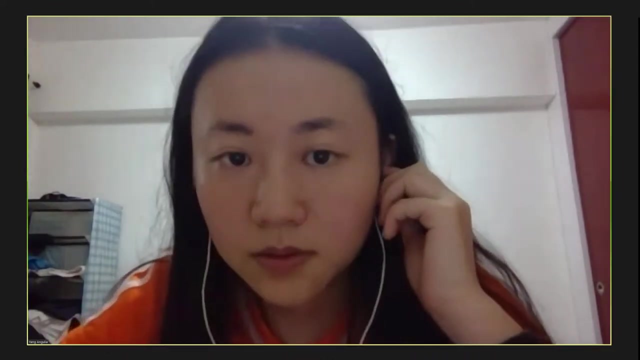 you all to join this. thank you, bye, bye, bye. i say too, okay, i think say through is ave angulia, so uh, yeah, so i'll be dropping off. hello, hello, yeah, i. i said I think Setu is away, so I think I'll end the meeting okay. 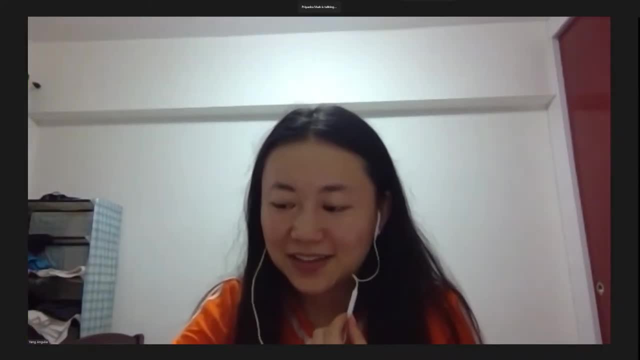 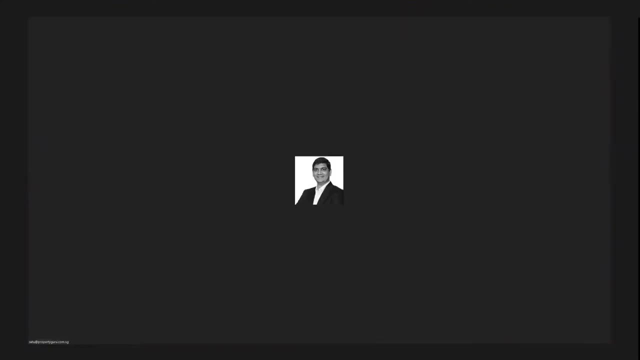